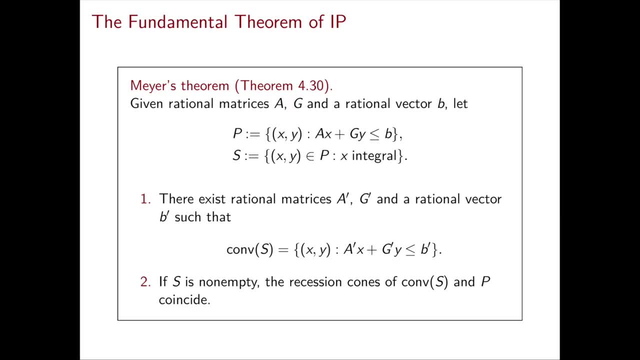 used, as I mentioned back in chapter one when we discussed that solving a mixed integer linear programming problem reduces to solve a linear programming problem over the convex hull of S, exactly because convex hull of S is a rational polyhedron. So essentially we're using the results that we're going to prove. So here is the statement of Mayer's: 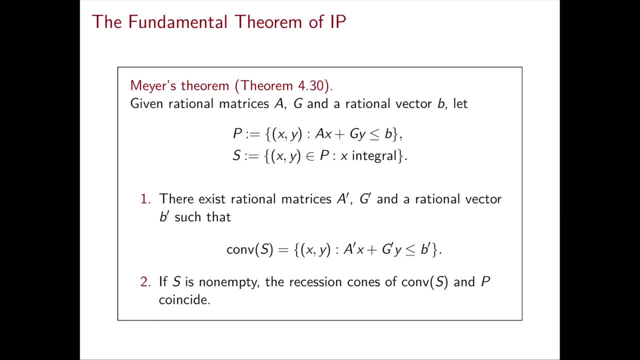 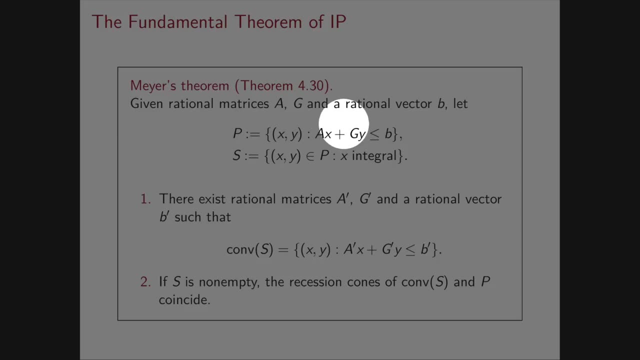 theorem, which is the fundamental theorem of integer programming. It says that if you're given rational data, so again A, G and B are rational. then let's look at the polyhedron P given by AX, X plus GY, less than or equal to B, and at the corresponding mixed integer linear set, which 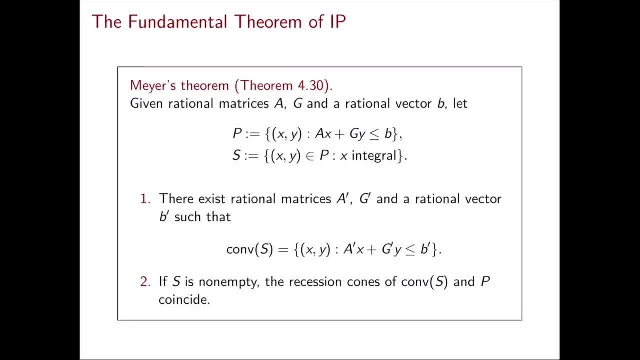 is the set of points in P with X integral. Then two things. So first, convex is a rational polyhedron, So namely convex can be written as a set of XY with A prime, X plus G prime, Y, less than or equal to B prime, for some A prime, G prime and B prime which are rational. 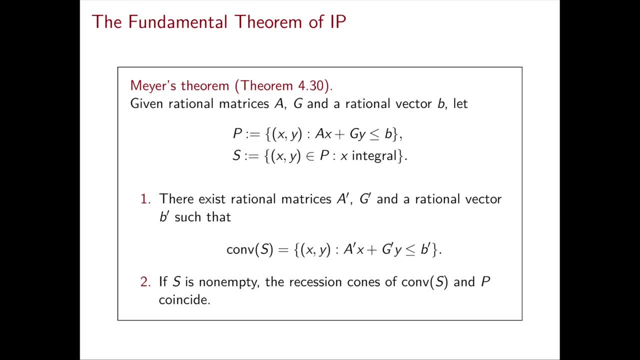 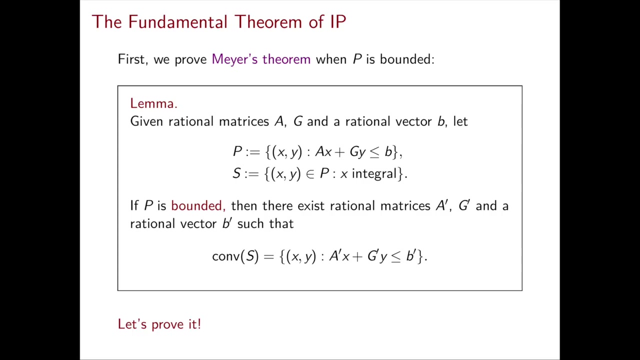 Furthermore, this theorem also shows that if the set S is non-empty, then the recession cones of P and of cone S coincide. So the first task in this section is to prove this theorem, And the first thing we want to do is prove it in an easier setting, and that is when P is bounded. So we're going. 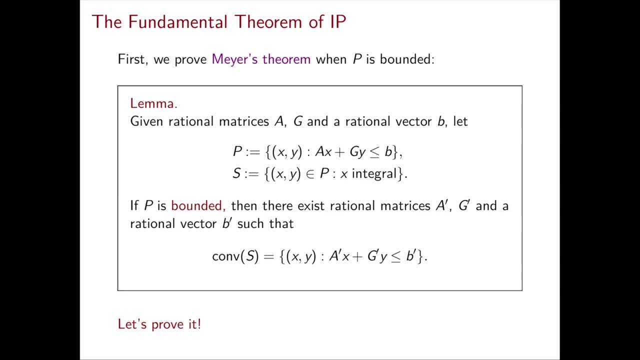 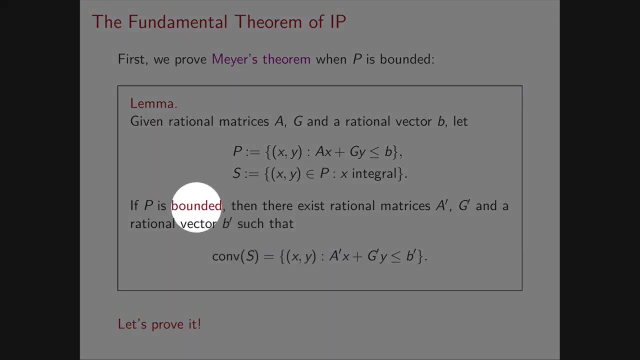 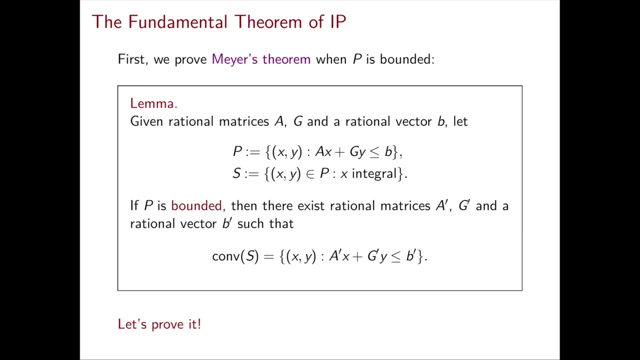 to be proving this lemma. It's very similar to the theorem we've just stated, So the setup is the same: We have P and S as before. Now we're assuming, though, that P is bounded, and we're claiming that convex is a rational polyhedron, which, of course, will be a rational polytope at this. 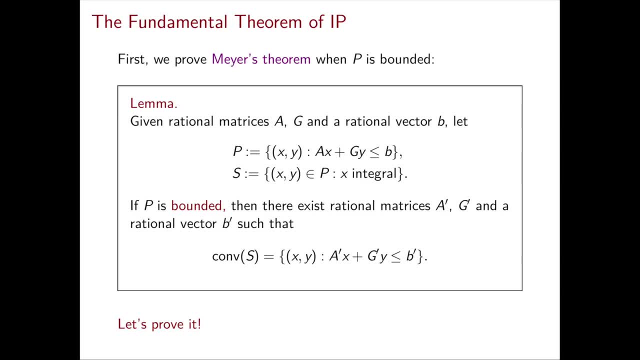 point. So what's the difference with the previous theorem? We're assuming P bounded and also we are not showing the second part, essentially, of the theorem. This is just the first part. I mean, the first and second parts of the previous theorem are gone, and now we're saying that. 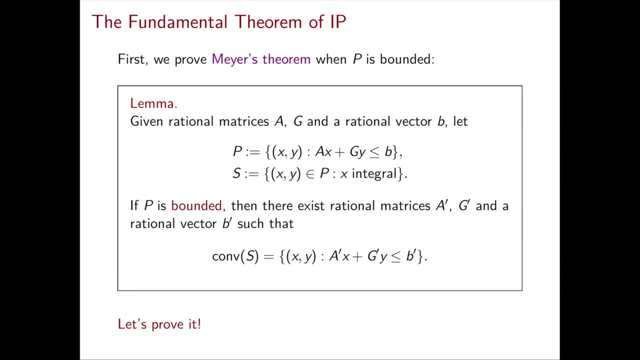 we don't need the second point. It's not the second part of the theorem. Why? Because in this case, if P is bounded, clearly, the recession cone of P and cone S will be just the origin. Good, So then let's prove this lemma. 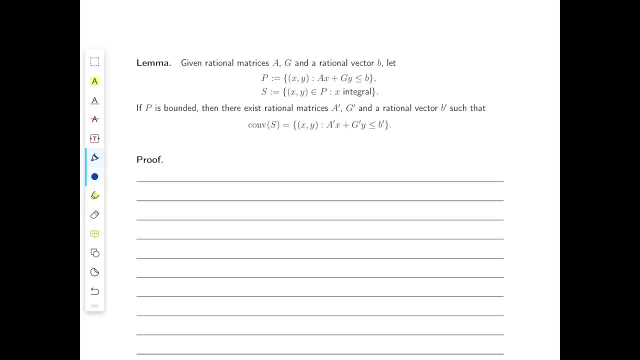 So how are we going to prove this lemma? So the idea here is to subdivide the set capital S into two. We just do the same thing. So you've got this into different sets based on the component x of the point. so essentially, if you think about 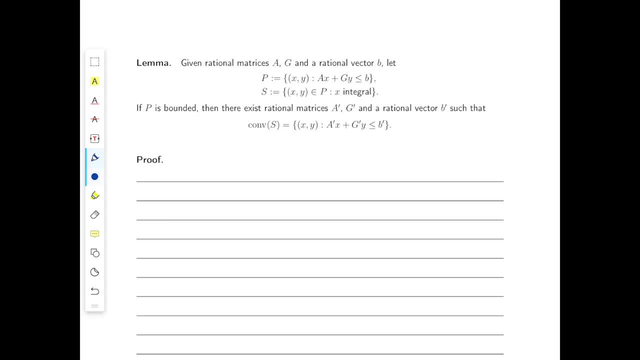 the set of points in capital S with the same x, which of course has to be integral. this will form a different polytope inside p, which is then the convex hull of its vertices. now, if we take these vertices for every polytope of this type that we can derive the convex hull, 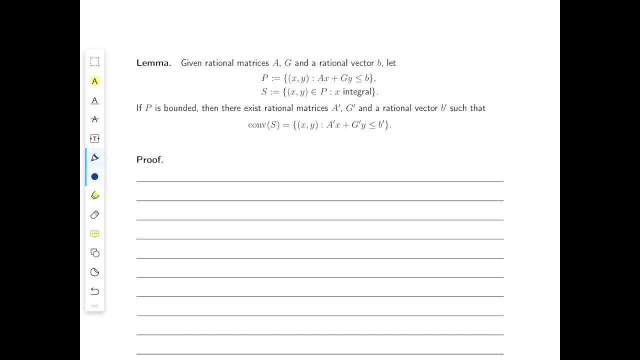 of all of these vertices will be exactly the convex hull of S, and this is just the whole idea that we're going to use to prove this lemma. so let's start, and the first thing we want to do is define the set of possible axes for which there exists a point with that capital S. 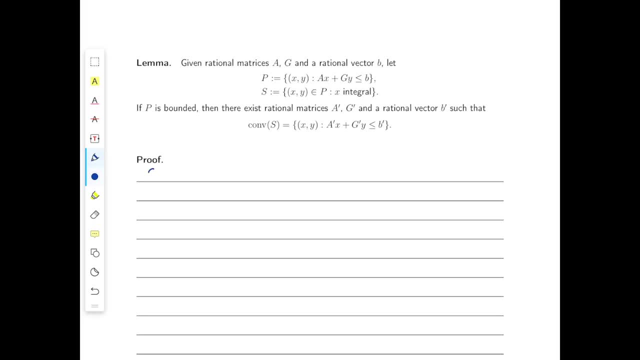 x in capital S. So let me write it. Since T is a polytope, the set capital X, defined as the set of x's for which there exists a y with x, y in S, is finite. So here we have defined this set capital X and also notice that it's finite. Next we want to use this: 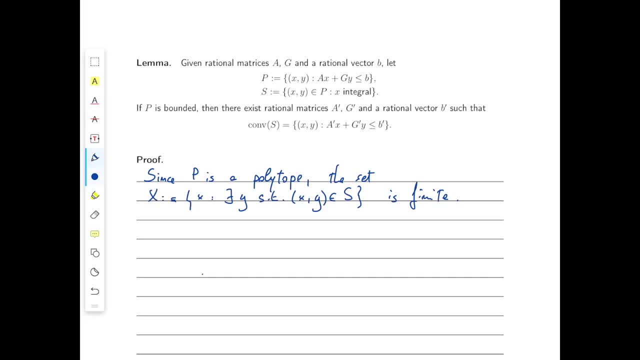 set capital X to partition, the set capital S based on the set capital X, The component x of the points. So let me write for fixed x-bar in capital X, the set- let's call it S- x-bar, defined as the set of points, x-bar y, for which x-bar y is in S. So what? 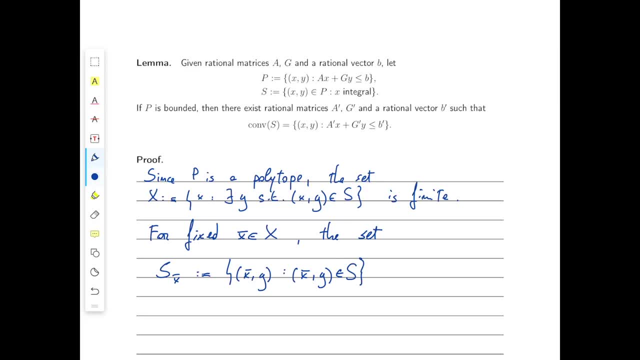 I want to say is that this capital X is finite, The set capital Y is a rational polytope. Well, maybe it's not obvious if we see it based on the definition we just gave, but everything we really need to notice is that 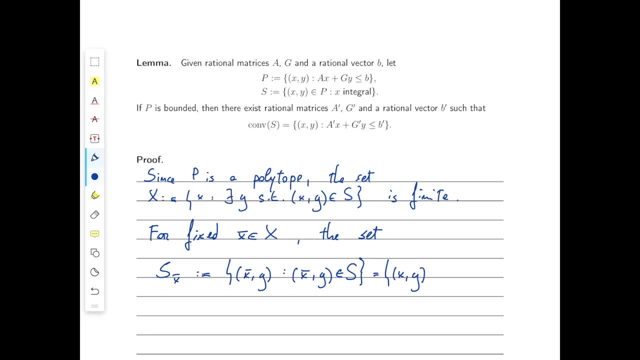 this can be written equivalently as a set of points- x, y- in P, with x equal to x-bar. So now this is clearly a polytope, because, well, it's contained in P and it's given by the inequalities defined in P and the additional equalities, x equal to x-bar. So 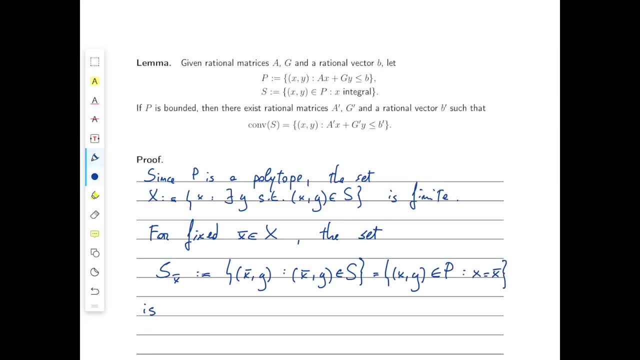 then we can write that this is a rational polytope, So in particular it's a convex hull of its vertices. Let's call the set of its vertices vx-bar, which are of course rational Good. so at this point we can just take the union of all these sets, and we're taking the. 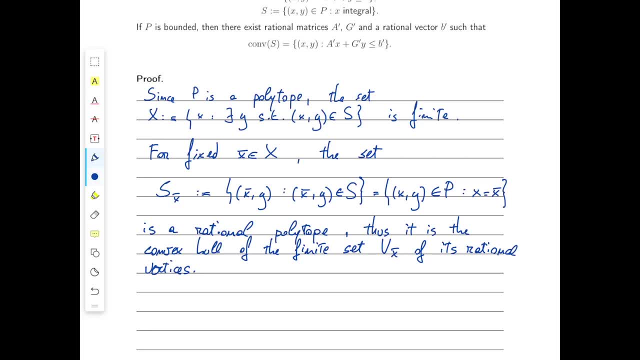 union of a finitely many finite sets. so we obtain a finite set again. So let's write it, Since a capital X is finite. also, let's define a set v as the union for x-bar in capital X of the x-bar, and it's finite. 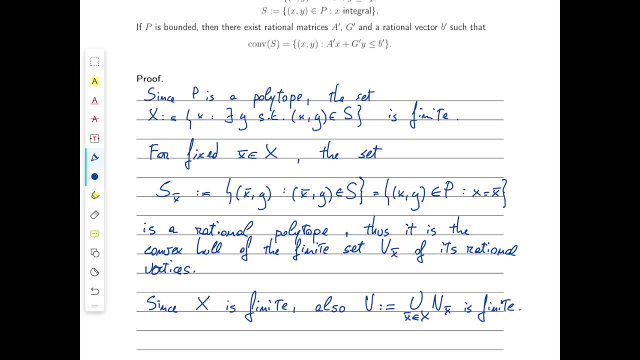 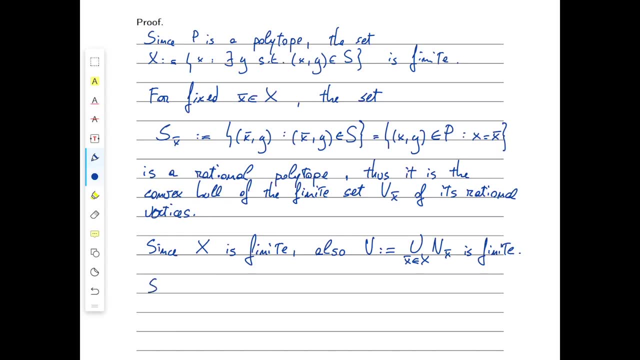 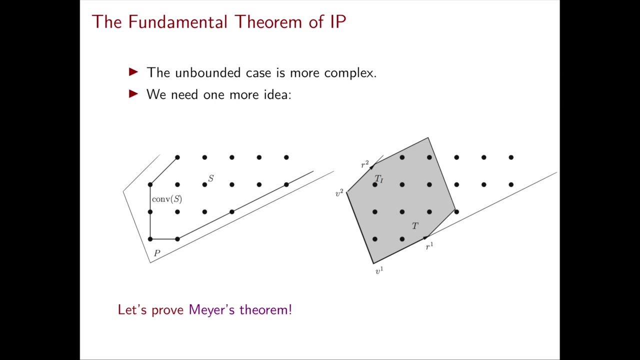 Good, and we're done, because at this point the convex hull of S is exactly the convex hull of capital V. So let me write it here: Since cong S equal cong V, we have that cong S is a rational polytope. And this concludes our proof. Now the general case of Maier's theorem is: 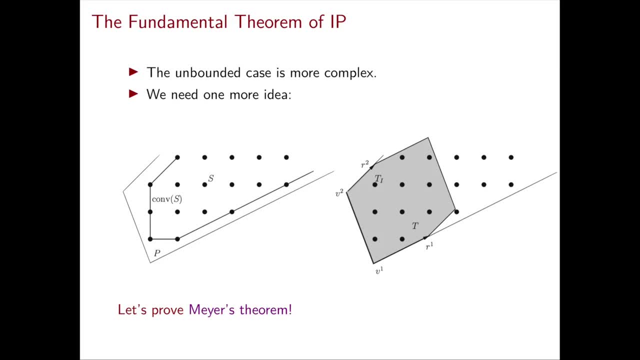 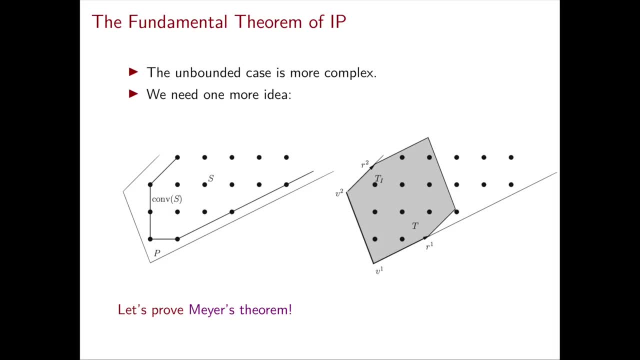 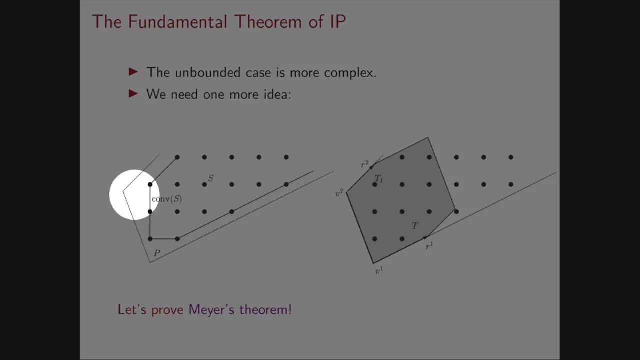 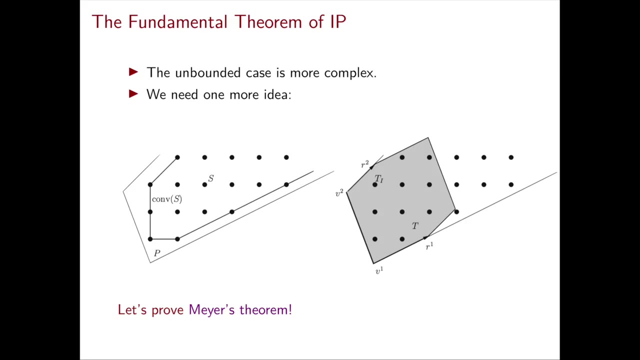 Which are the vertices of the convex hull of S. In general, P is described by Minkowski-Weil as the convex combination of its vertices- in this case, these two guys over here- plus a conic combination of its rays- in this case, these two guys over here- And, of course, the 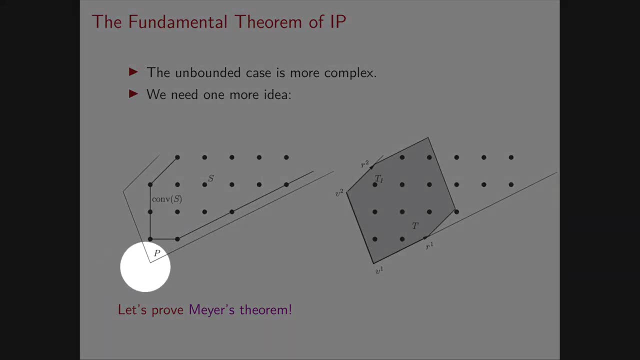 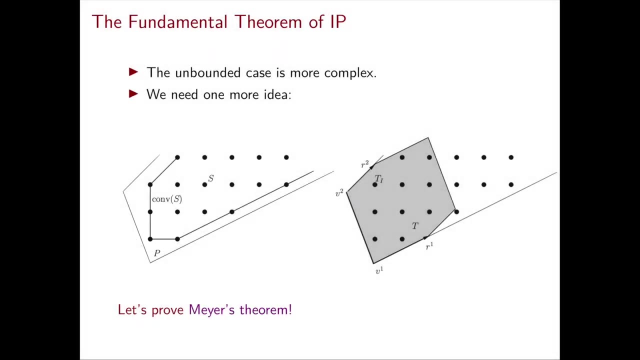 convex hull of the vertices of P. So this segment doesn't necessarily contain all the vertices of convex. In fact, in this case it doesn't contain any of them them because they're just somewhere inside the polyhedron. However, what we're going, 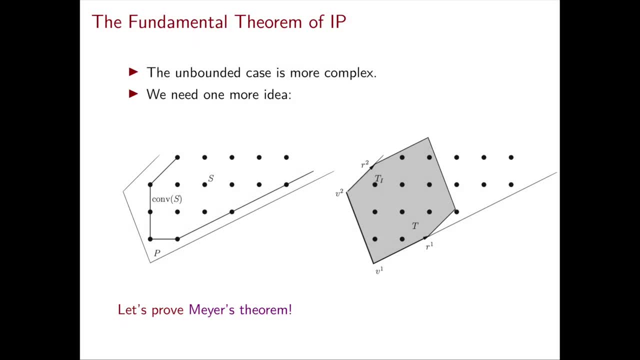 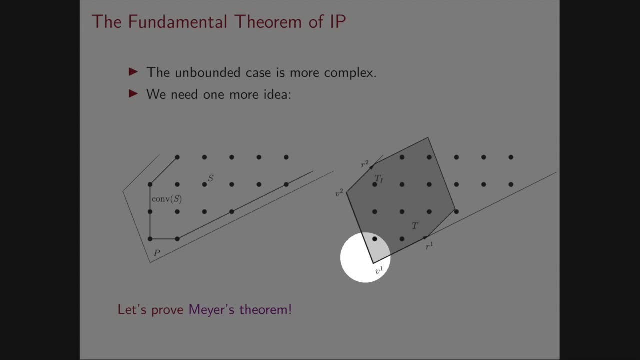 to show, which is clear from this picture, is that all the vertices of convex, in fact, are quite close to the convex hull of V1 and V2.. Essentially, what we have to do is take the convex hull of V1 and V2 and add to them the extreme rays of the recession cone And 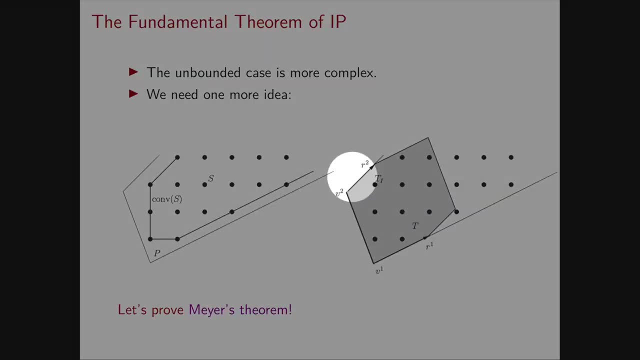 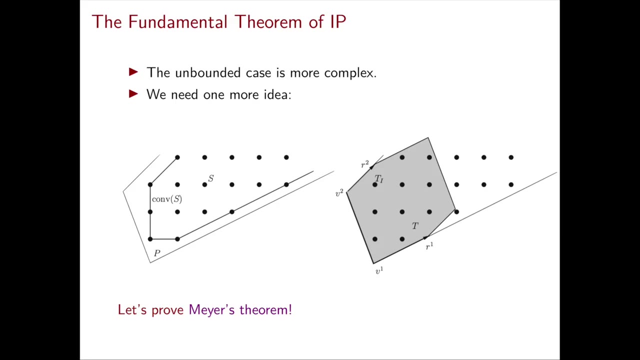 of course, rays are only defined up to scaling, and here we just need to take any integral scaling of such rays. Good, So essentially, this observation will allow us to prove this theorem. Of course, it's still unclear why or how, but let's keep in mind this picture. 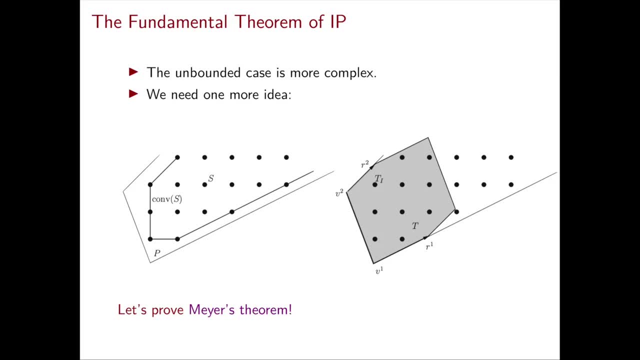 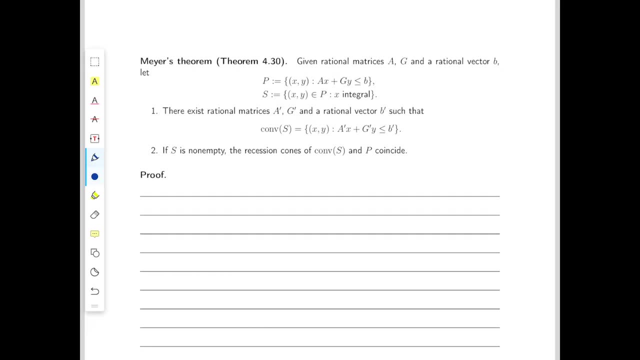 because it will definitely help us in the proof in order to understand the proof. Good, So let's get then to the proof By theorem 3.37, and that's what we call the decomposition theorem. for polyhedra, There exists vertices: V1,, V2, V3, V4, V5,, V6,, V7,, V8,, V9,, V10,, V11,, V12,, V13,, V14,, V15,, V16,, V16,. 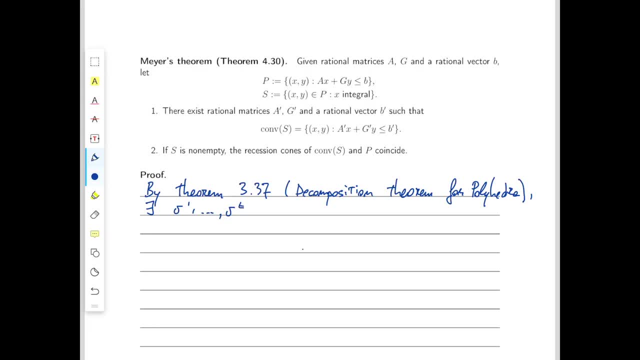 V17, V18,, V19, V20,, V21,, V22,, V23, V23, I mean they're not necessarily vertices, points V1, Vt until R1, Rq, such that V. 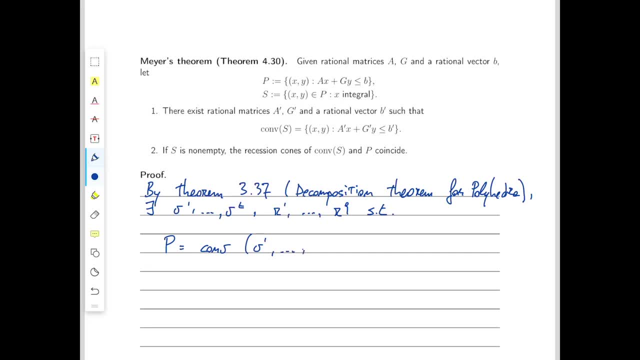 is the convex hull of V1, Vt plus the conical of R1, Rq. So now we know here that V could have a linearity space. so these are not necessarily vertices, they're just this v1- vt, they're just. 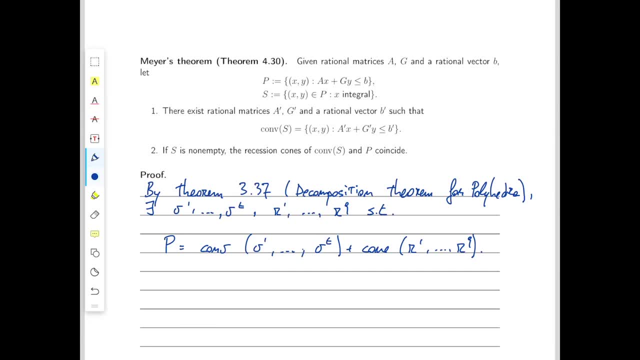 generally points in the minimal faces of p, but i strongly recommend you keep as a running example in your mind the picture we've seen before. so i or at least appointed the polyhedron which has vertices to make things a little bit clearer in your head. so the first thing is to notice is that all these 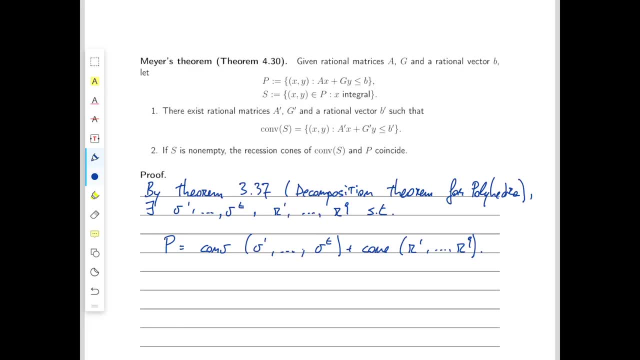 vectors that we have just written are rational, because the system defining p is rational and, furthermore, then we can scale the extreme rays in order to make them integral. so let's write it like this: good, now we have everything we need to define the truncation of p, which was the gray region. 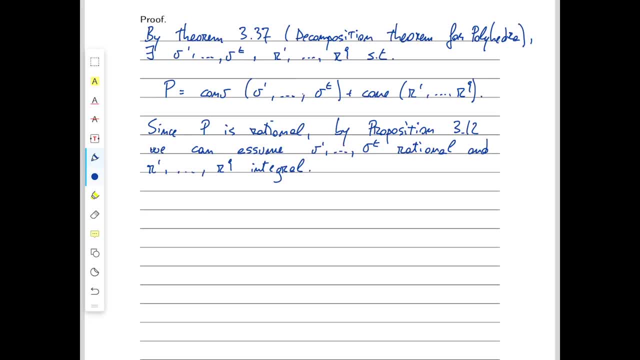 in the picture before. so this region that we essentially conjecture contains all the vertices of converse, so let's write it down. consider the truncation of p, defined by the vectors x, y. that can be written as convex combination of this v i's plus, not really, let's say, an almost conic combination of the. 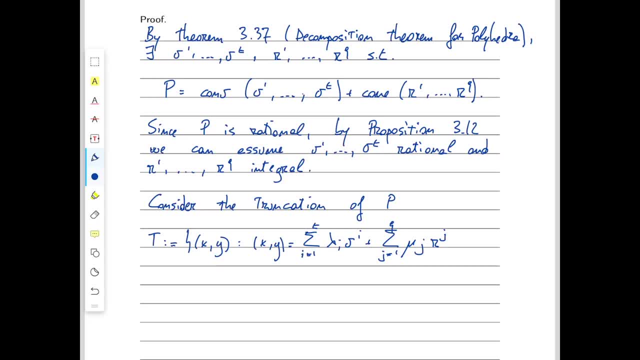 rays. so this is our vector x, y and we just need to write conditions on the lambdas and mu's. so lambdas are just convex combinations. so sum of the lambda i equal one right, equal one until t and lambda greater than or equal to zero. and then what about mu? 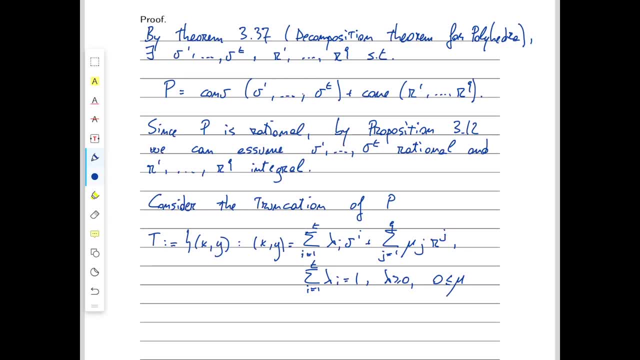 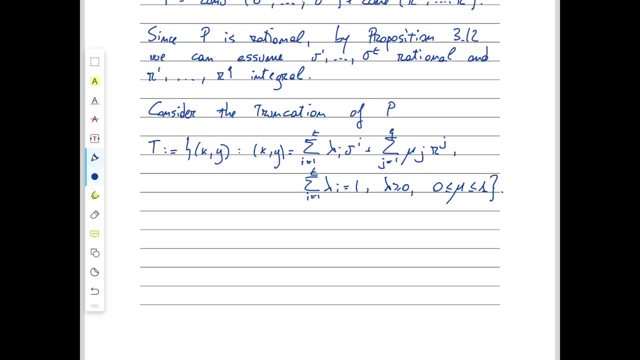 if this was just a conic combination, we would have just mu greater than or equal to zero. but here we add less than or equal to one. so that's how we truncate the polytope. good, now, this is also a rational polyhedron. why? because all the data describing the system 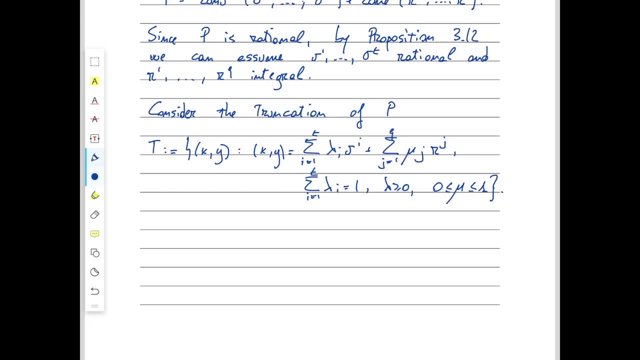 is rational, so right, all the vi's and rj's are rational. so this is a rational polyhedron. so let me write it. since v1, vt, and and r1, rq are rational, t is a rational polyhedron. moreover, t is a polytope. 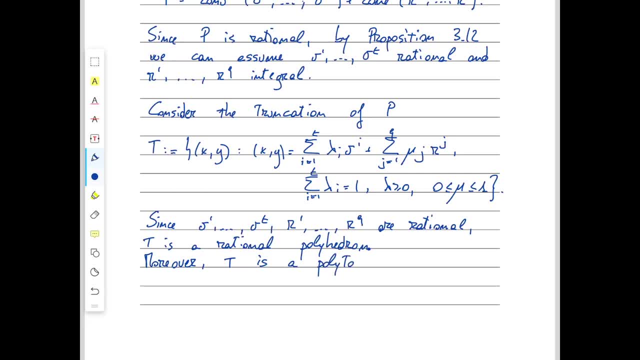 why is that so, question for you. why exactly figure out all the details? so let me give you the idea. essentially, look at the points x, y that we just have in the set t. they are the points that you can write in this way. good, now we will have a little demonstration of that in. 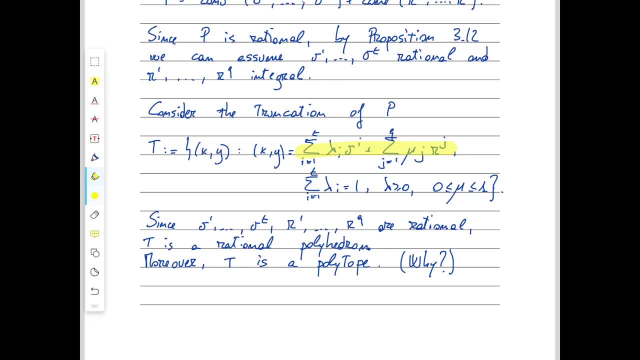 a moment now you see that all the multipliers are bounded between 0 and 1 because, well, mu is clearly written, mu between 0 and 1. what about lambda? well, it's greater than or equal to 0 and also upper bounded by 1 because of the equality sum of the. 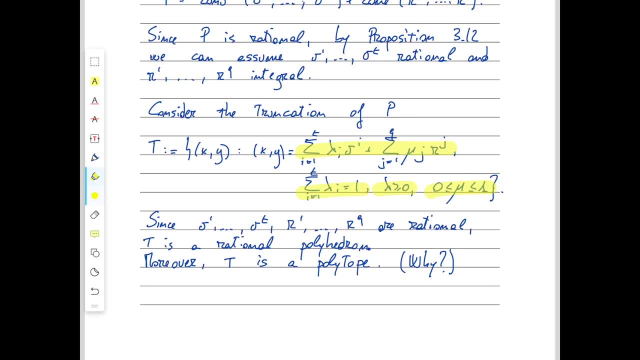 lambda i is equal to 1, so this is just a. these are bounded combinations of vectors, of finitely many vectors, so they must be bounded as well. this is just of course idea. you should figure out a formally correct proof. good, so at this point we are ready to define the two sets corresponding. one corresponding to: 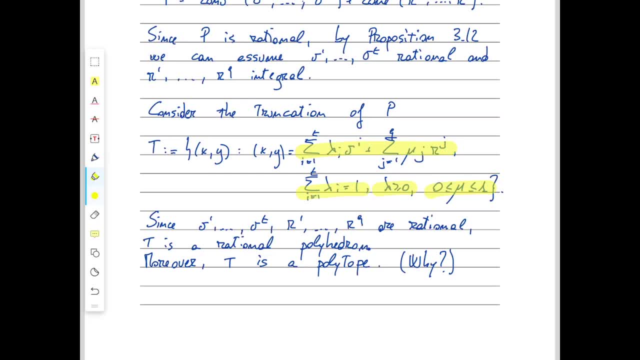 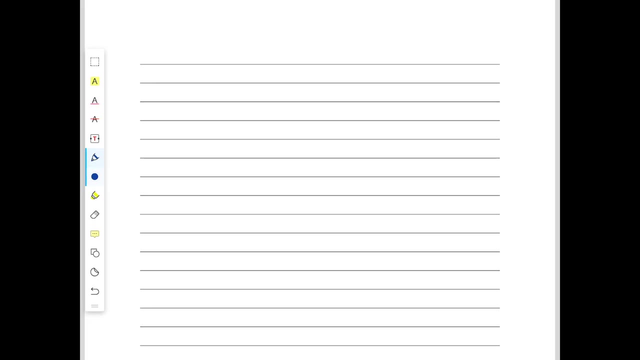 T and one corresponding to the recession cone of P, that allow us to break down S into the Minkowski sum of two different sets. so let's write these definitions. let- oops, let- TI be defined as just a points in T with X integral. so the set of XY in T. 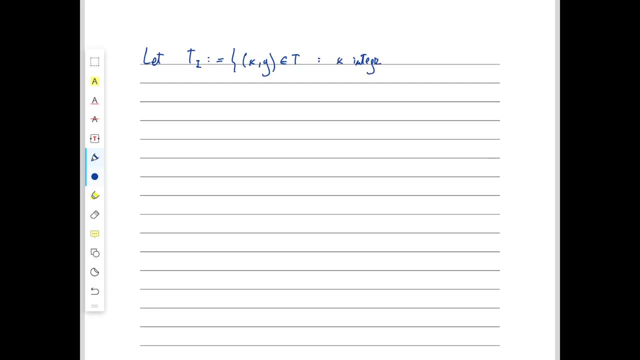 such that X integral and RI so RI. it's a type of set that we've never really seen before. this is the sum of the mu, J, RJ, for J equal to 1 until Q. so so far so good and nothing new. but what I want to? 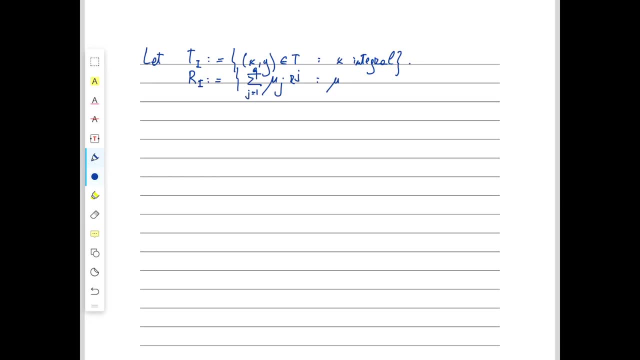 enforce here is that mu is not only greater than or equal to 0, but it's also integral. so these are just integer combinations of our arrays, RJ's. what we want to show is that S is equal to TI plus RI. so this will take us a little bit of work to do, and the first thing we do is 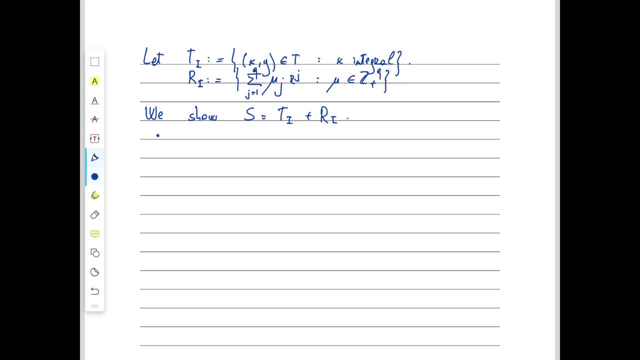 so the easy containment he is the following: clearly: s is the superset of TI plus RI. so why is that? well, pick any point in T: I, this is in T, and with X integral, and now we add it to it vector in Ri. this is a vector in the recession cone of P, so we're still. 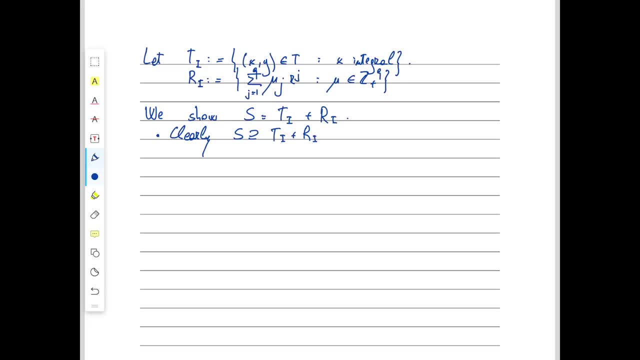 inside P, for sure, and it's also integral. so we're summing a vector in Ti which has already X integral with a vector that is fully integral. so the X component of this vector will remain fully integral, and that's how. that's the reason why the sum of these points is not only in P but also in S. Good, so this. 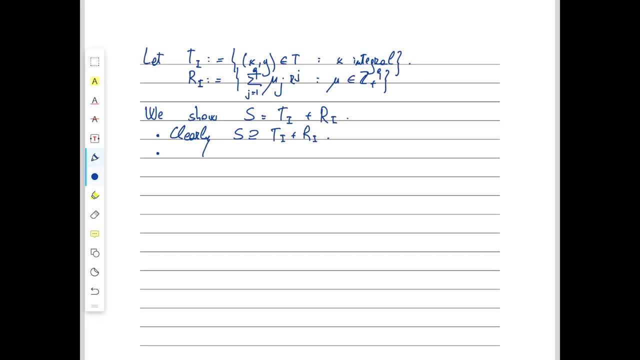 is easy. if you want to fully understand it, please write down the foolproof that I have somewhat said and let's instead focus on the reverse inclusion. it's a little bit more difficult, so for the reverse inclusion, pick a point: X, bar, Y, bar in S you want to show it is in. 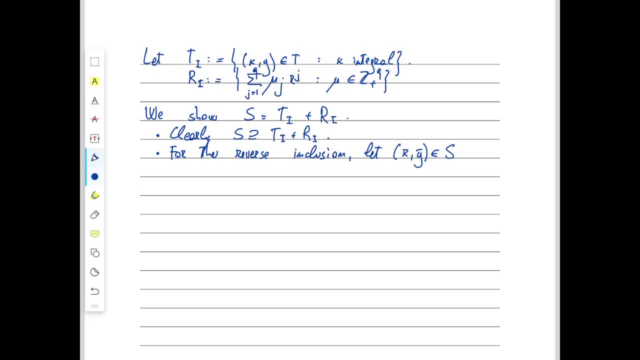 S Ti plus Ri. so essentially, what I want to do is explicitly write X bar Y bar as the sum of these two vectors. So what do we know? we know that X bar Y bar is in P and this immediately implies that we can write X bar Y bar as a combination of: 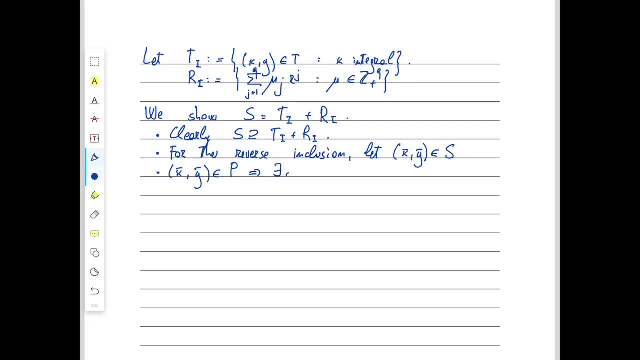 our Vi's and our J's, so let's write it there: X is lambda mu greater than R, than or equal to zero, with the sum of the lambda i for i. that goes from 1 to t equal to 1, such that x bar y bar equal to the sum of lambda i, v, i. 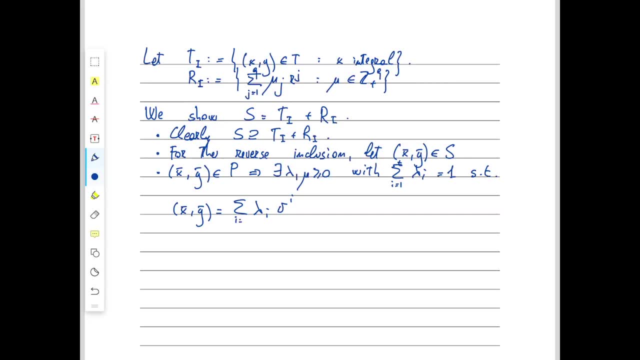 as always, for i that goes from 1 to t, plus sum for j that goes from 1 until q of the mu j, r, j. okay, now we're going to use the sums to define the two vectors, that one will be in ti and one in ri, so i'm going to keep the convex combination as it is. 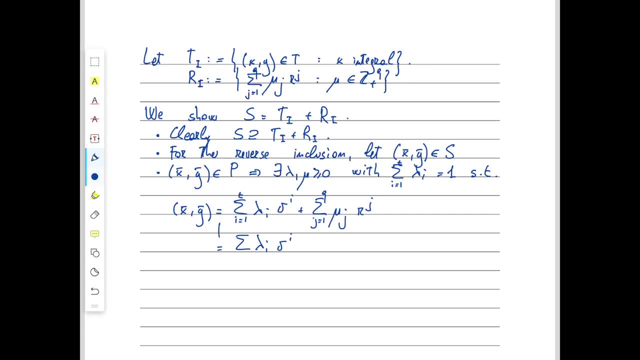 i, okay, i can leave the sums without the indices. you know what i mean. so i'm going to keep the convex combination as it is. and now for the conning combination, i'm breaking down. i'm breaking it down in an obvious way, in such a way that the first point i obtain is in the truncated polyhedron. so what do i need? 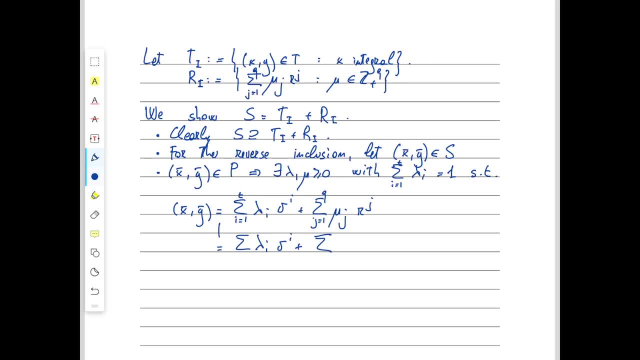 i need the mu at most one, so i artificially make it at most one by taking mu j minus the floor of mu j times rj, and of course i am left with what's left, and this is exactly the floor of mu j times rj. good, and now i define this first part to be, let's call it, x, prime, y, prime. 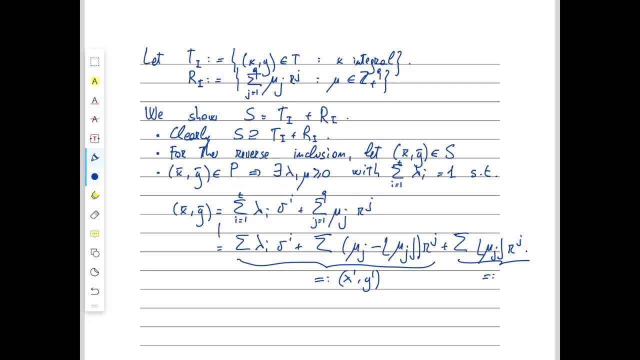 and the second part. i define it to be r. let's call it r. so what can we say? let's focus on r. let's put in r. so, because i want to put a so speed to the environment, which is simpler. so look at R. this is by definition in RI, right? this is an. 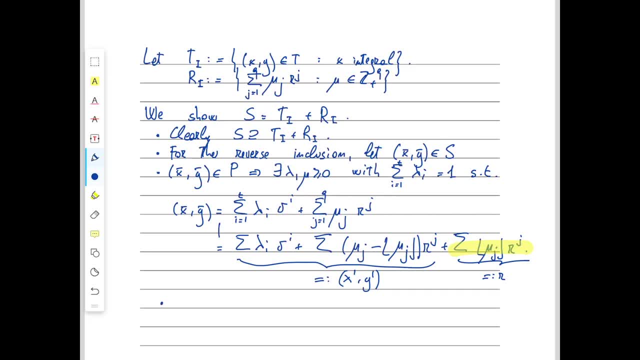 integer combination of the RJ. so immediately, by definition, R is in RI. so what about then? X prime, Y prime. so the first thing we notice is that the multiplier on the J's is between 0 and 1, so which implies that it's in T. so let's. 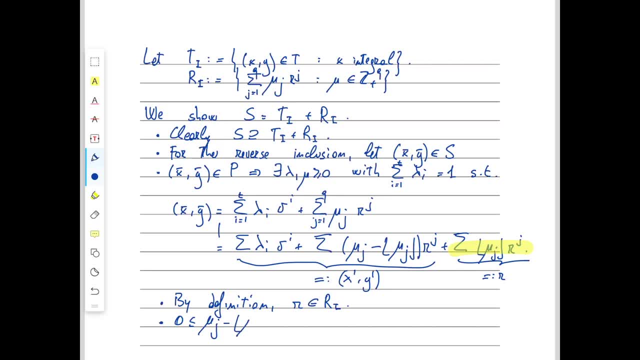 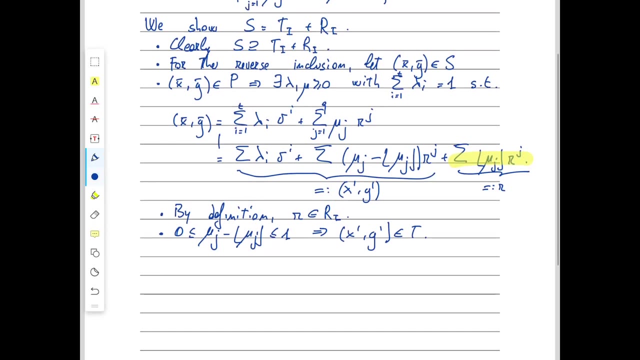 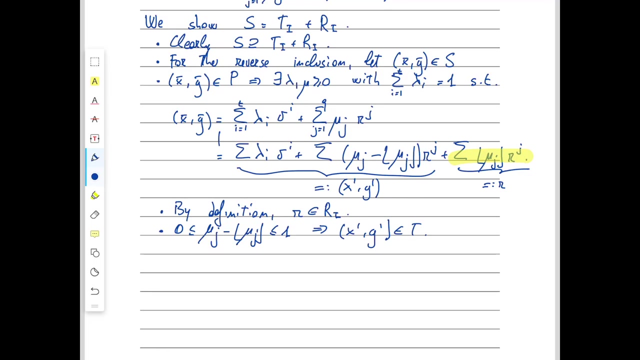 write it: mu J minus the floor of mu J is between 0 and 1, which implies X prime, Y prime is in T now. so, if you remember, we want to claim actually that this point is in TI, so we want to show that X prime is integral. so what is exactly X prime, using the equality that? 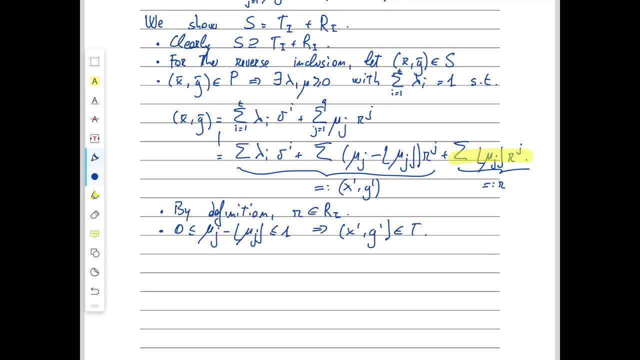 we just have above. here we have that X prime is X bar minus the components of R, which correspond to the X space, but R is integral. therefore X prime will be integral as well. so let's write X bar and R integral imply X prime integral. so we have X prime, Y prime in TI and this concludes. 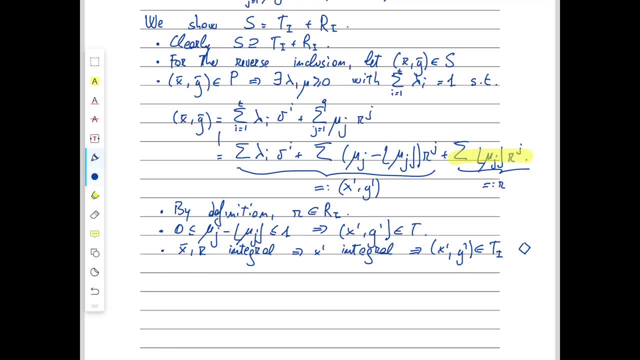 our claim, so we're finally shown this- that S is equal to TI plus RI, and so we can continue now and use this, this equality, and everything we're going to do now is take the convex hull of this set, so we take the convex hull of S. remember, that's what the theorem is. 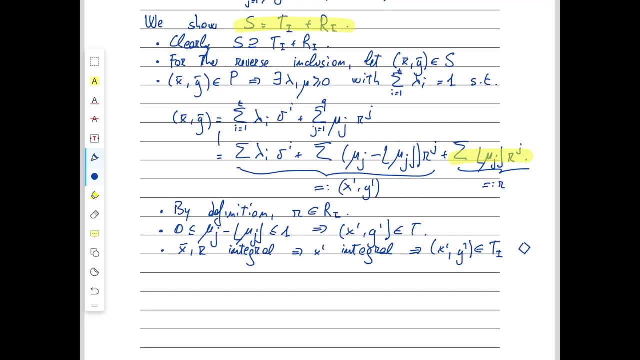 about. we want to discuss the convex hull of S, and so that's the convex hull of TI plus RI, and the Minkowski sum can be brought out of the convex hull. this is an exercise you have in one of your assignment sheets, so let me write it. 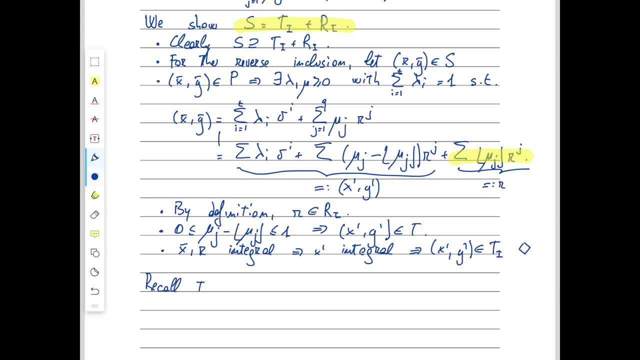 recall that the convex hull of a Minkowski sum is the Minkowski sum of the convex hulls and if you want to look at it, it is on your site- critical. so what the Minkowski sum of the convex hull of T really means is that we know that S is equal to TI plus RI. 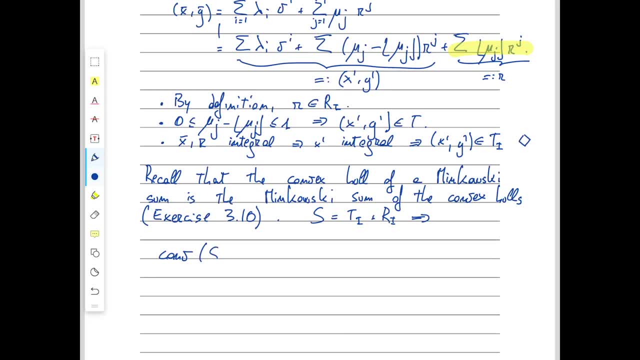 this, exactamente, is what this set applies. so we'll at the very end of the F word and say to each value is that these two, those are the contrails- lives on our vector aspect. we know that these conv ti and conv ri. Again, the simpler one to understand is conv of ri, because 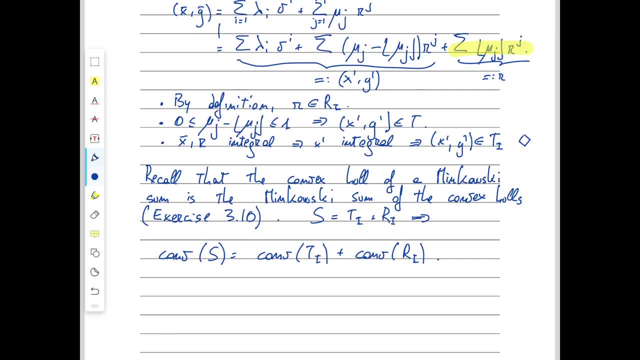 it's exactly the cone defined by the vertices r1 until rq. So clearly, conv of ri is equal to the cone of r1 until rq. And then what do we know instead about the conv of ti? Well, we know that t is a polytope. 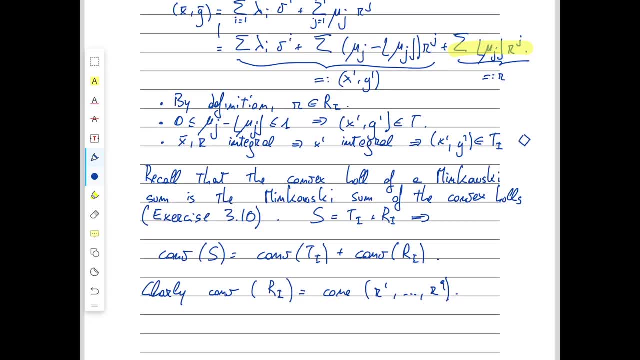 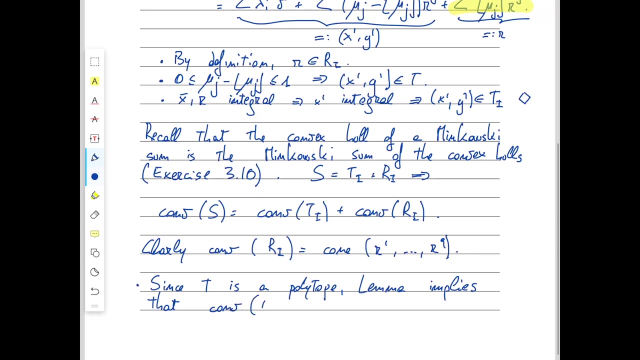 so now we can just apply the lemma that we've shown before this theorem. So because we have the assumption that the set is bounded, So let's say, since t is a polytope, lemma implies that conv of ti is a rational polytope. 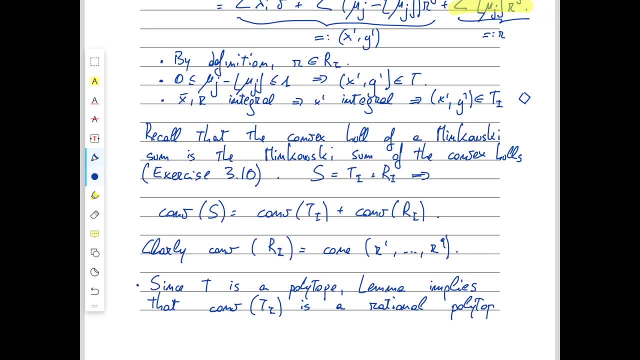 Good. So at this point we have a cone and a rational polytope, And so, by Minkowski-Weil, conv? s is a rational polyhedron, and also, since conv? ti is bounded, its recession cone is exactly conv of ri. So let's conclude. 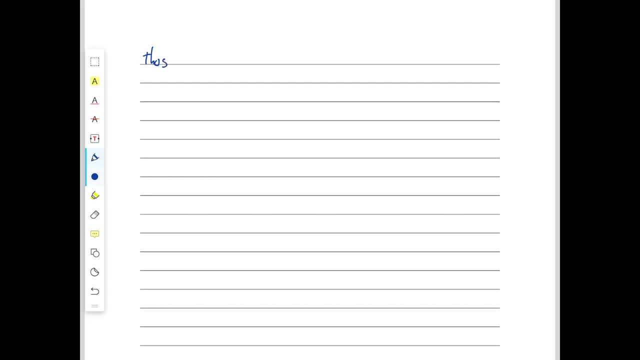 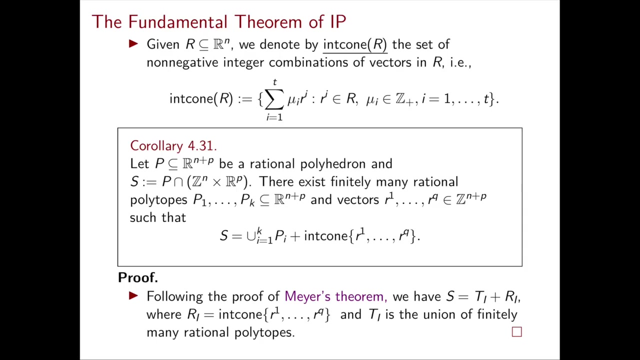 Thus conv? s is a rational polyhedron having the same recession cone as P. And this concludes our proof. In the proof of Maier's theorem we have used this type of cone, which is an integer combination of a bunch of vectors. So here I just want to define formally: 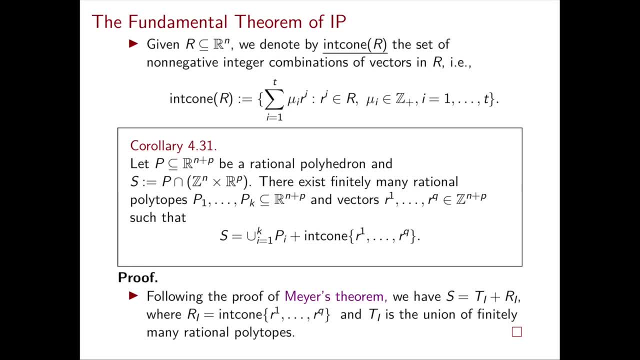 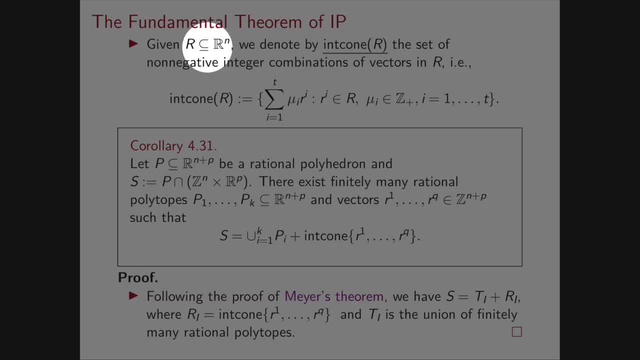 I mean, I just wanted to introduce some notation for this type of cone so that we can use them later. So we're given a set of vectors- capital R, let's say- and we denote by int cone, which stands for I con r, The of r that we looked at exactly in the proof. So what? 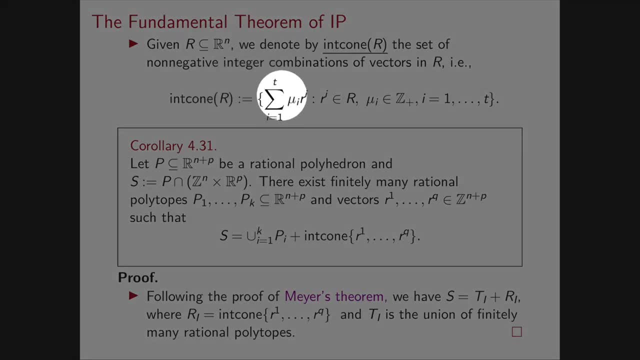 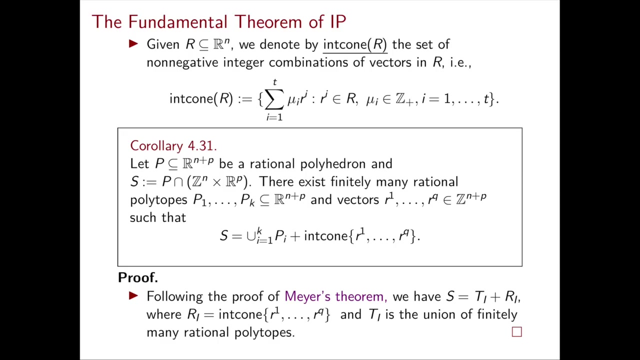 was this. Well, we, we take any combination of the vectors ri in the set capital R, but only with non-negative integer coefficients. Good, So then we can immediately write the following corollary: It doesn't look particularly interesting now, but we're going to. 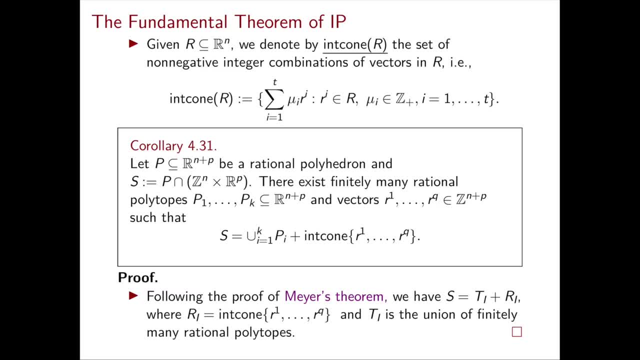 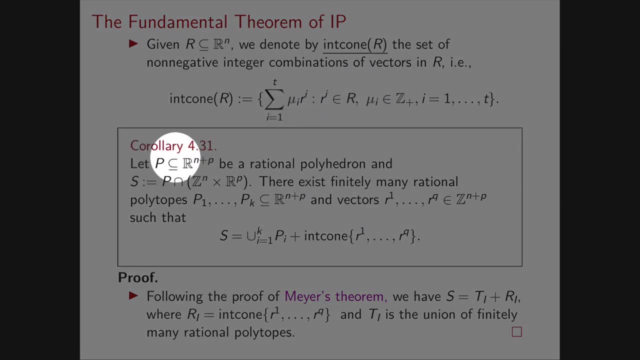 use it later, later on in this chapter, for a representability result. so we're definitely going to need it and it follows directly from the proof, from what we have seen in the proof of Maier's theorem. so let's read through this: we have the same setting as Maier's theorem, so we have a rational polyhedron and we 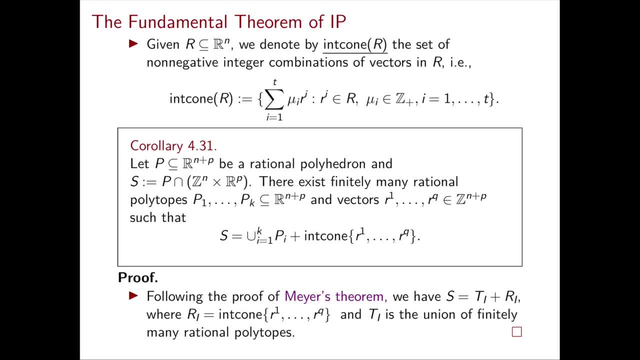 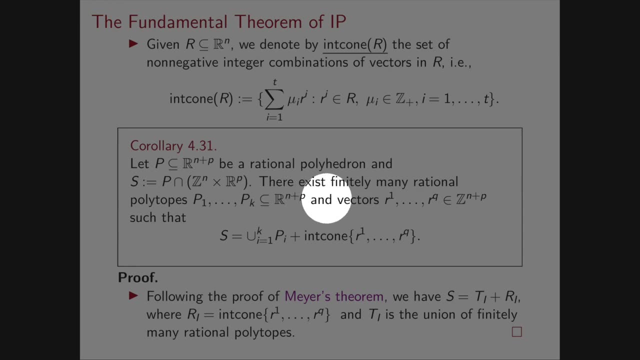 look at the mixed integer points inside P and we denote those by S, and what this corollary says is that there exists finitely many rational polytopes- P1 until Pk- in the same space, and some vectors- R1 until Rq, such that the set 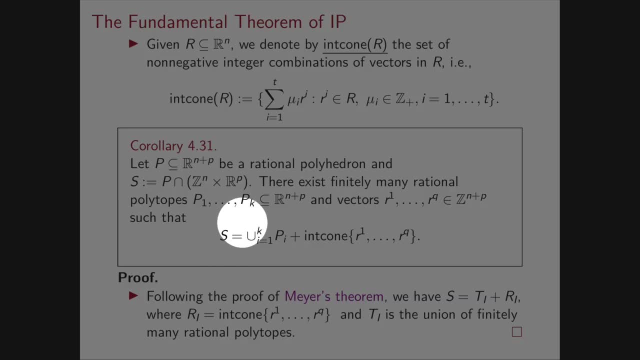 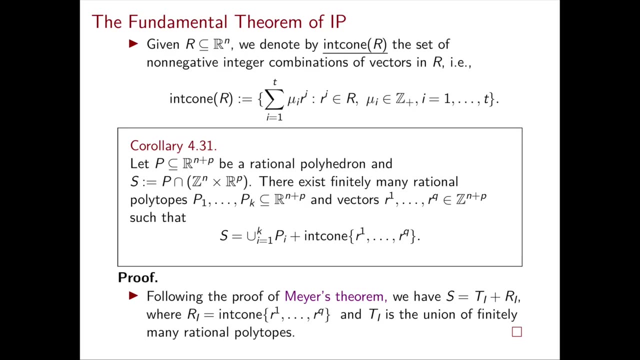 capital S of feasible points is exactly the union of this finitely many rational polytopes plus the integer cone of these integer vectors. and how can we prove this? well, we've seen that because in the proof of Maier's theorem we wrote down this: 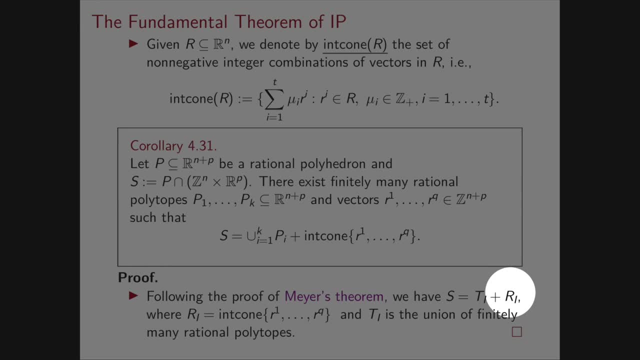 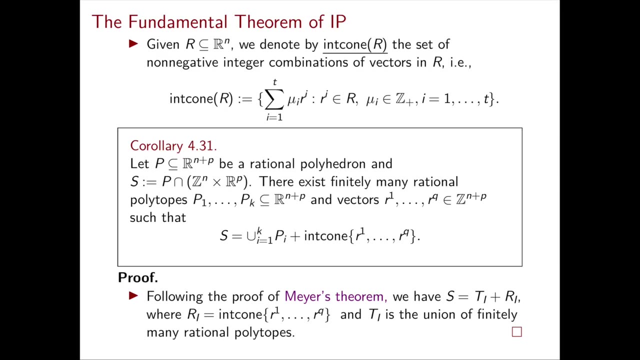 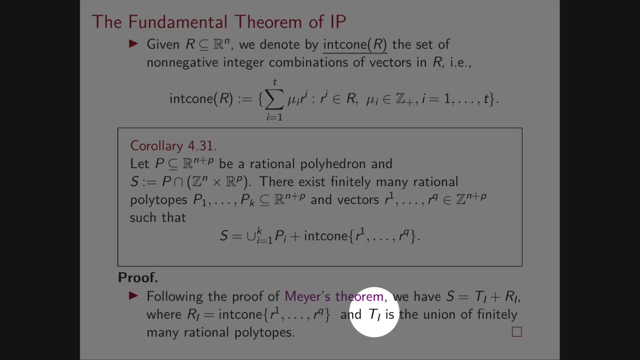 general set S as Ti plus Ri, where Ri was exactly the integer cone of R1 until Rq. we just didn't call it this way because we hadn't introduced this notation yet, and Ti was instead the union of finitely many rational polytopes. 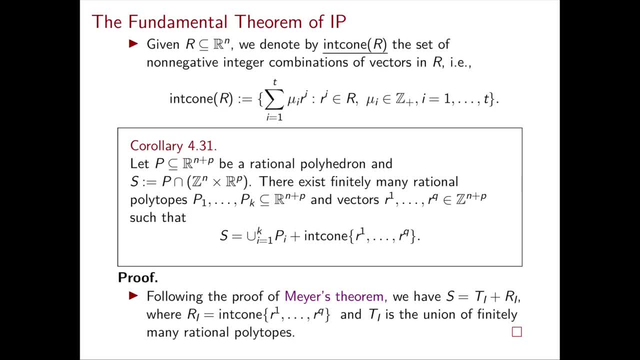 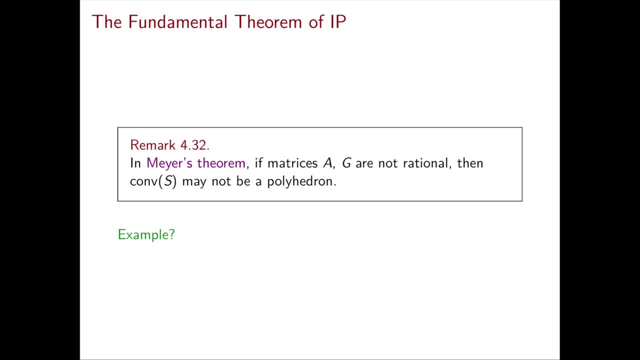 as we've seen in the proof. so great, let's keep, then, in mind this corollary so that we can refer to it later. good, so the next thing I want to mention is the rationality assumption in Maier's theorem. so we had the assumption in: 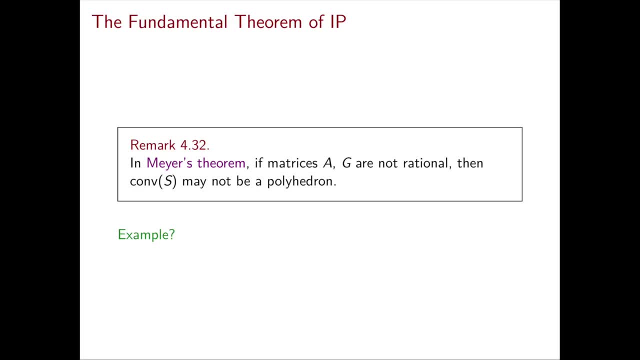 Maier's theorem that all the data is rational and in fact what you can check is that this assumption is fundamental for the theorem to hold. and well, one might wonder if just dropping the rationality assumption in Maier's theorem results in just obtaining that convass is a polyhedron and not necessarily a Vi. 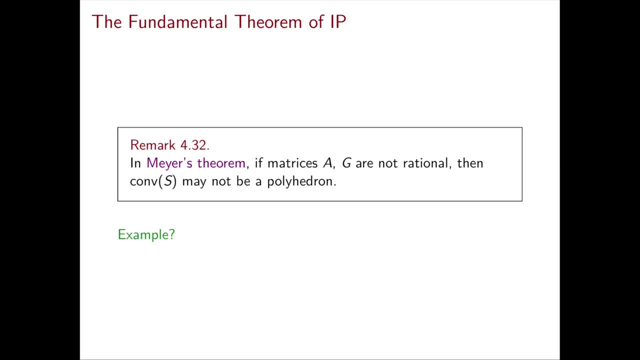 so essentially you one may wonder if you can just remove Vi every time it appears in the statement of Maier's theorem. just cross out this word and see if the result still holds. and in fact it's not true. if you remove the rationality assumption even just from Maier's theorem process, you can remove just the rationality assumption, even just from Maier's theorem. don't move. quite simply, this is not true. Locker's Theoremppy Theorem. why did Cup? 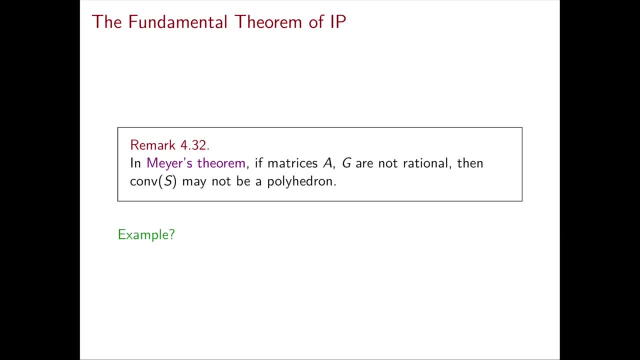 A and G, then you might obtain something that is not even polyhedral, and here this is a very good exercise for you: think about possibilities and try to understand how convests might look like if A and G can be indeed irrational- and essentially you can see examples of convests not being a polyhedron already. 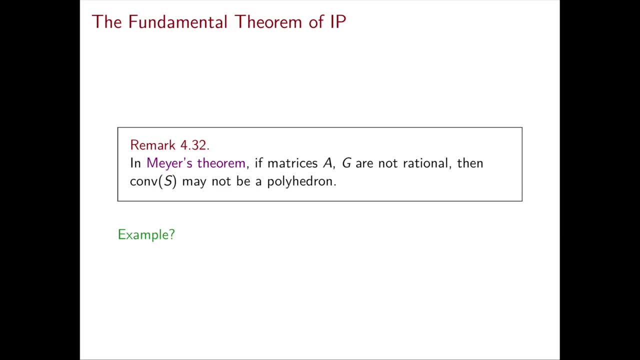 in dimension two. that's definitely good enough for you to think about counter-example this type of examples, and there are at least a couple of behaviors of the set convests that you can find out, so, for example, one: so in one of these two cases, the set convests will be essentially almost like a. 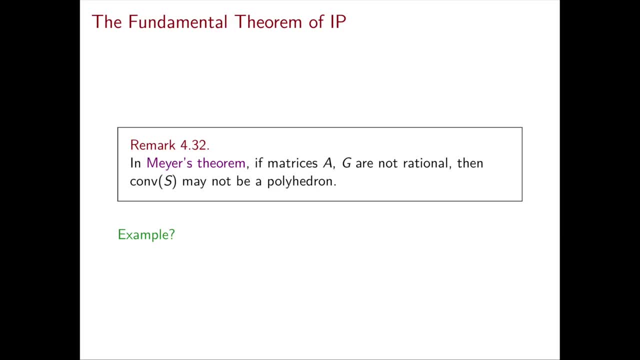 polyhedron. the only difference is that it will be missing some points on the boundary, and so, essentially, the closure of the set is a- in some cases- polyhedral, while the set convests is not a polyhedron. Another type of example that you can construct instead, which is kind of very different. the result is very. 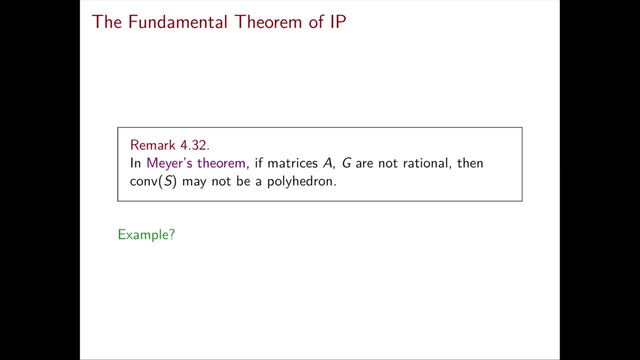 different is where convests is a closed set, but it's not a polyhedron, because it's actually defined by an infinite system of linear inequalities. so still is defined一樣 by linear inequalities, but infinitely many of them. So think about these two examples. 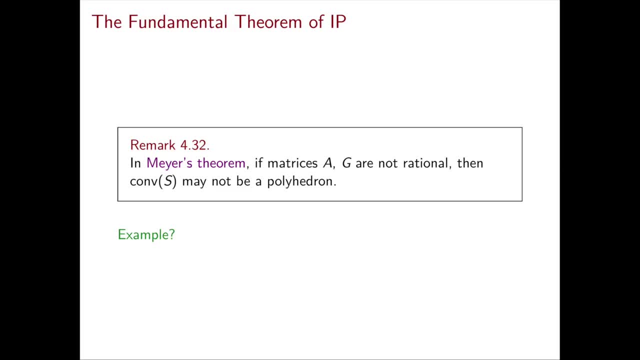 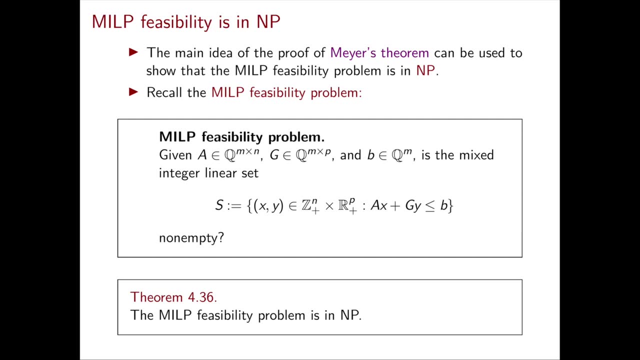 or maybe more. try to understand how this set convess might look like if you drop this rationality assumption. Good, So the next thing that I want to look at is the result that mixed integer linear programming feasibility is in NP, And why do I want to look at this result now? 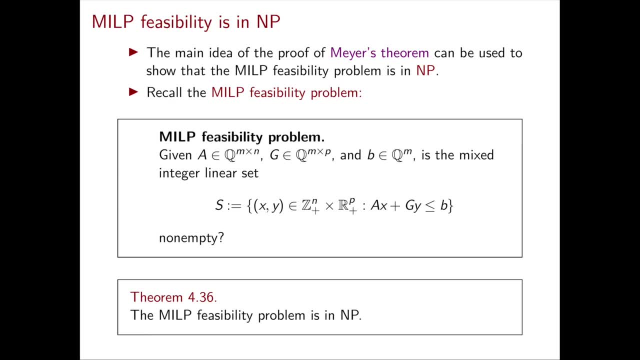 Because essentially the proof for this result is a modification of the proof of Maier's theorem. We just need to use a couple more ingredients which we've seen essentially already before. We discussed already the fact that mixed integer linear programming feasibility is in NP. 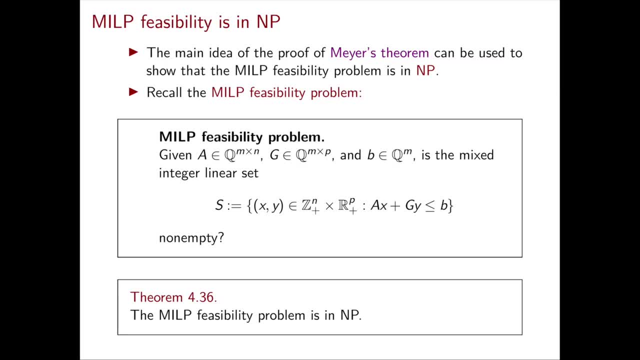 and I told you back in chapter 1 that it is an advanced result and we're going to see it later. so now it's the turn of the jump. So I am going to show you how it works and we'll see in the next class we'll explore how it works. Thank you very much for watching and see you next time. 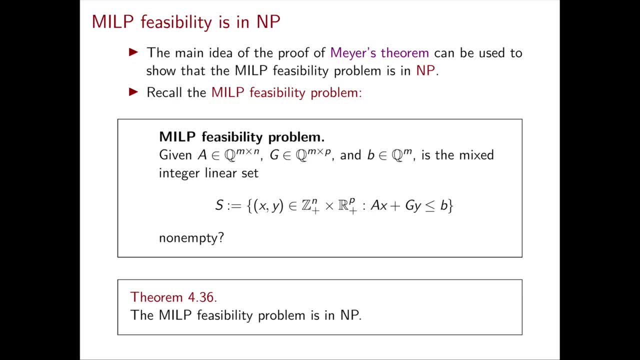 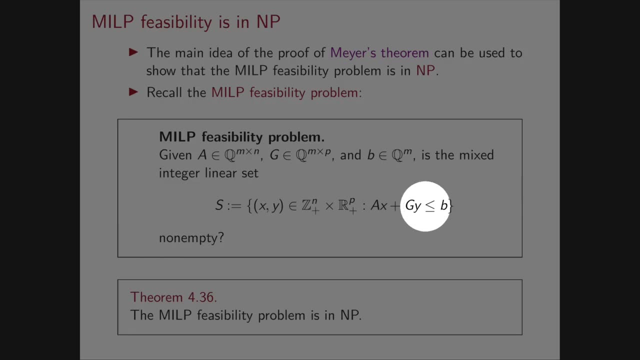 the time. So recall what is a mixed integer linear programming feasibility problem? Here it is. So we're given a rational data matrices- A, G and, right-hand side B, And as always, we look at the mixed integer linear set S, defined by AX plus GY, less than or equal to B, and everything is. 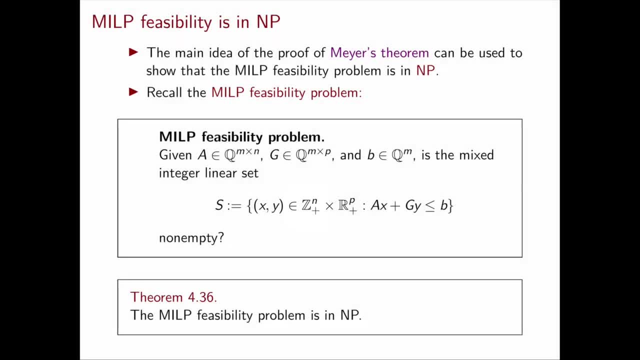 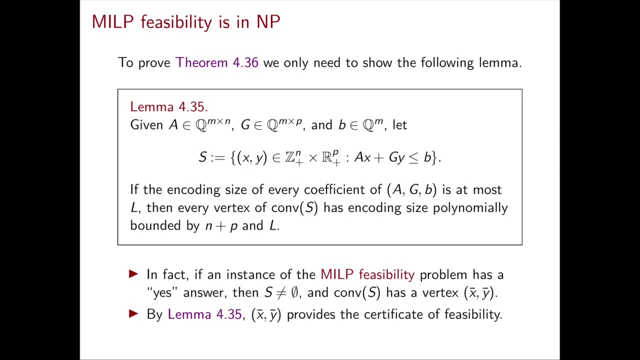 non-negative. And plus we also have that the X variables are integral. So the question is: is this set non-empty? And what we're going to show now is that this decision problem is in fact in NP. So almost all the results where some decision problem is in NP that we've seen. 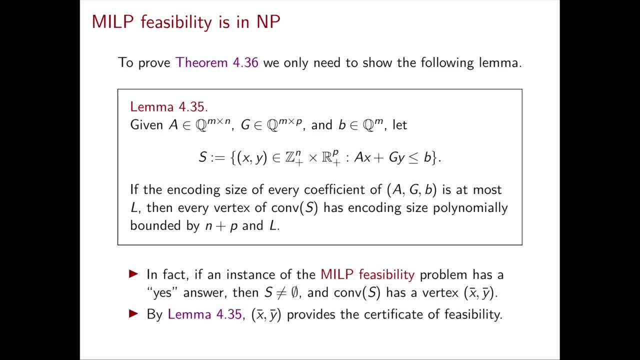 rely on giving as a polynomial certificate a point in the set. And so what did we do? for example, in linear programming, We discussed that a vertex serves as a certificate because it always has polynomial sides. So what we're going to show then, to prove that mixed integer linear programming feasibility is 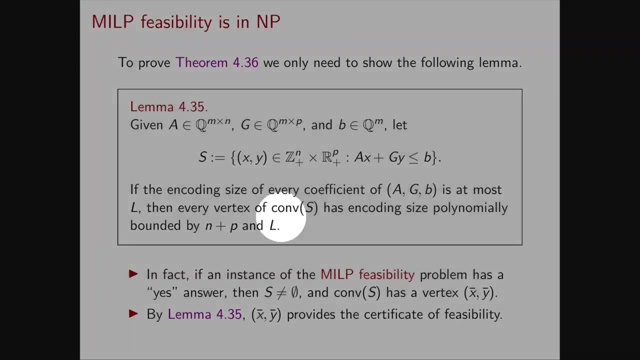 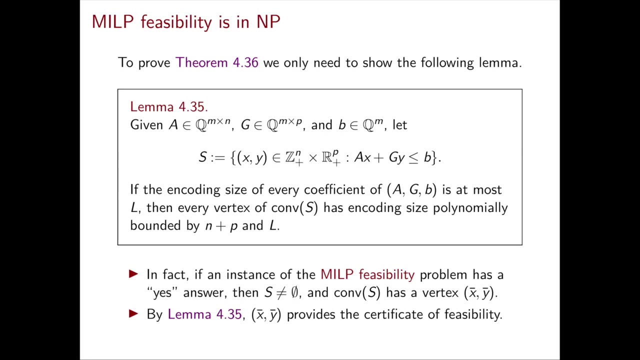 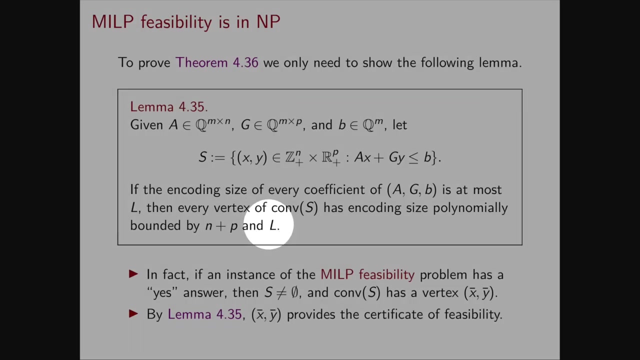 in NP is this lemma. So we look again at our set capital S as before, and we use capital L to denote the maximum encoding size of every coefficient in A, G and B. So then every vertex of conv S has encoding size polynomially bounded by N plus P and L. 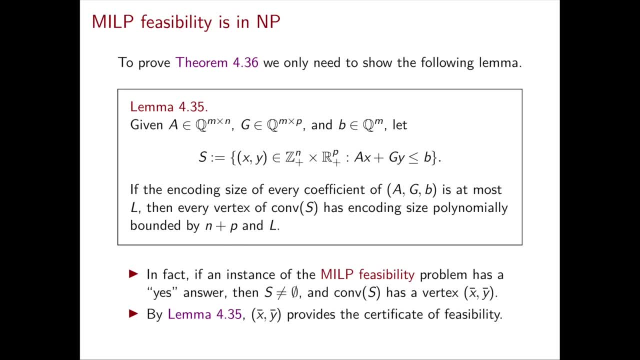 So in a sense very similar to the linear programming case. essentially, what you would expect In NP, a certificate was a vertex of the polyhedron, Now it's a vertex of the convex, all of feasible points. Of course we have to show this lemma, because why would this point? 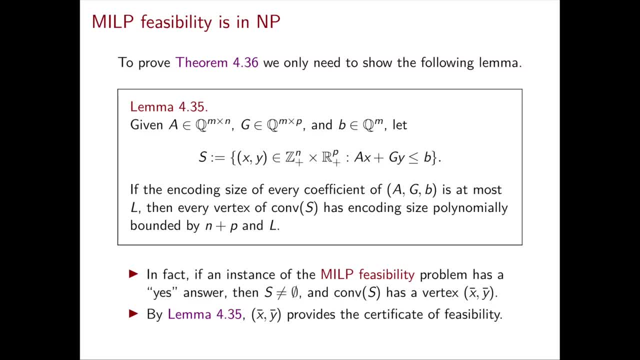 have a polynomial size. So we're going to show this lemma, because why would this point have a polynomial size? So this is, at the moment, unclear. that's what we have to show in this lemma. Once we have shown that lemma 4.35 is correct, then of course we know that the mixed integer 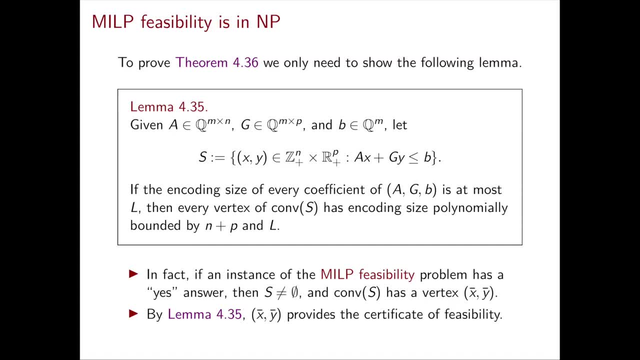 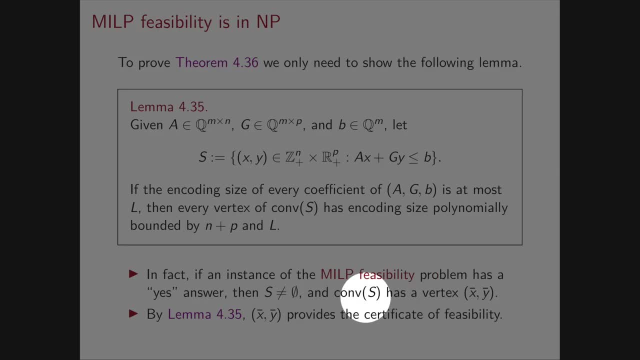 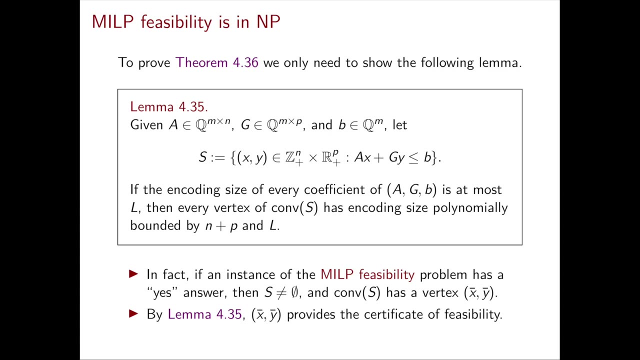 linear programming. feasibility is in NP because if the set is indeed non-empty then we can use a certificate. any vertex x by y bar of conv S. This is a certificate of feasibility because it has polynomial size and you can easily check. This is a certificate of feasibility because it has polynomial size and you can easily check. 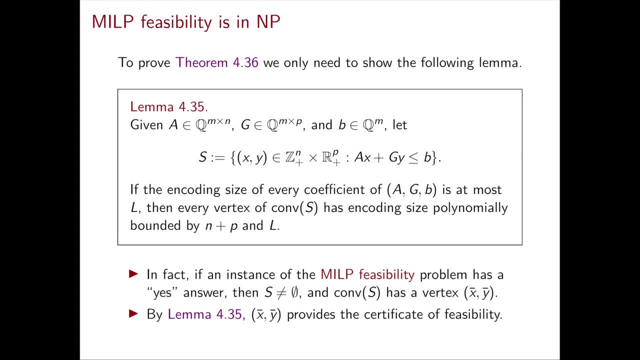 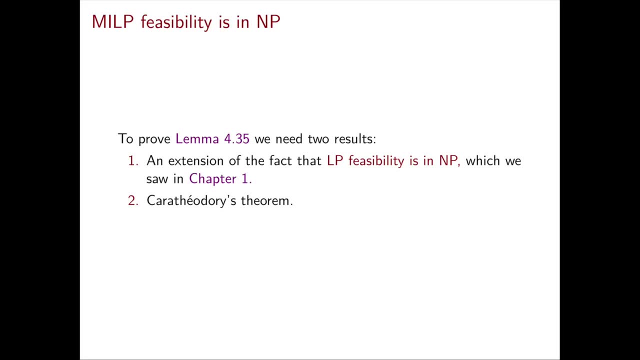 This is a certificate of feasibility, because it has polynomial size and you can easily check that it is indeed in capital S in polynomial time. Okay, so we need a couple of ingredients on top of the proof of Maier's theorem to show this lemma. 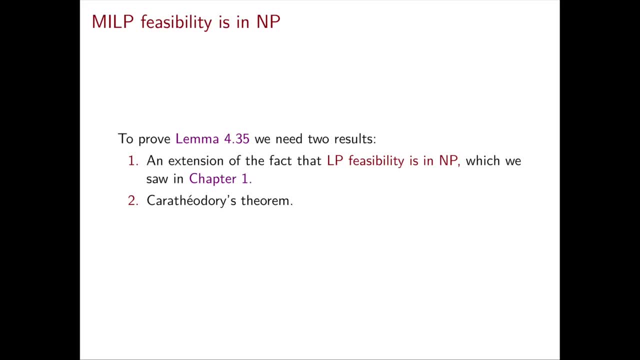 And these two results are: the first one an extension of the result that LP feasibility is in NP. This result- LP feasibility is in NP. we saw it already in chapter 1, we discussed it and we only focused on the vertices, of course, of the polyhedron. 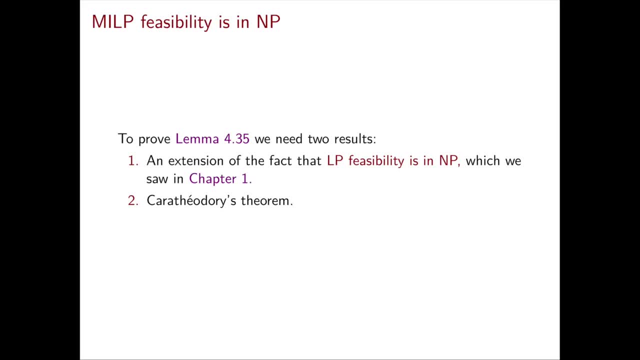 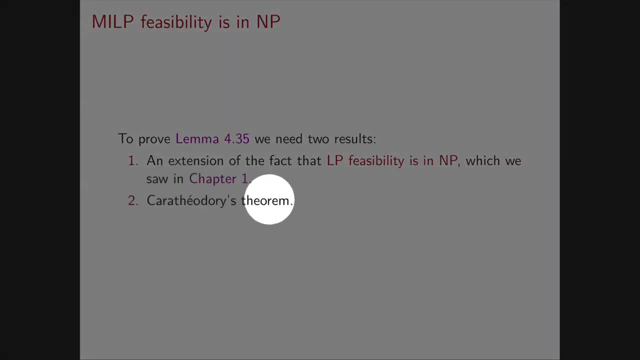 Here we only have to focus also, on top of that, on the extreme rays of the polyhedron. So that's the only difference. The other result is Karathiodorus' theorem, and we're just going to use it as we've already seen it. 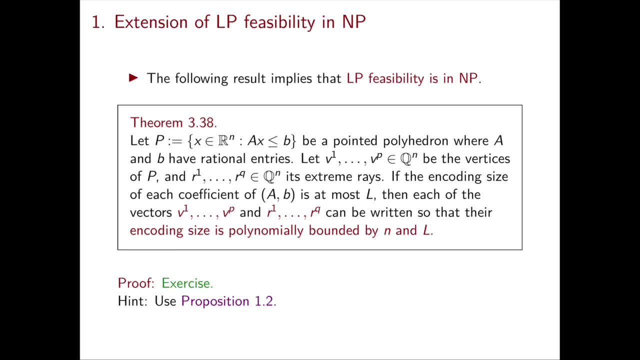 Okay, so this is the extension of LP feasibility. I'm now going to prove this result. it's an exercise and essentially it's the same exact argument that we used to prove that LP feasibility is in NP. The only thing is that you have to do essentially the same argument for the extreme rays. 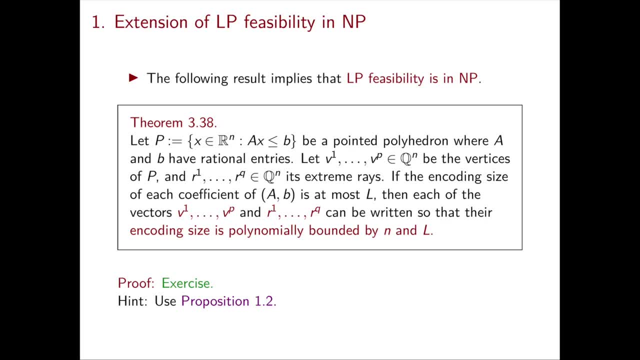 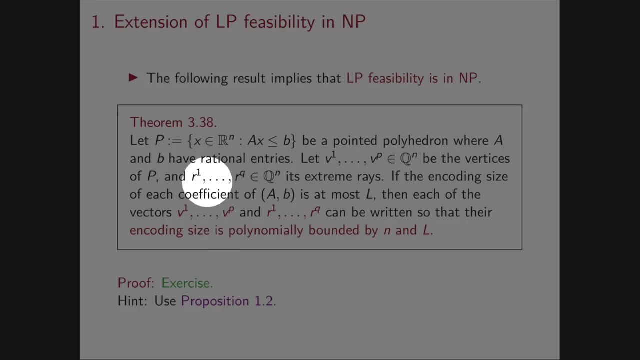 It's not exactly the same argument, because? well, because rays are defined only up to scaling. so it's a good exercise to figure this out And, yeah, essentially you need to do this. So we're going to use proposition 1.2, which is exactly the same we used for the vertices. 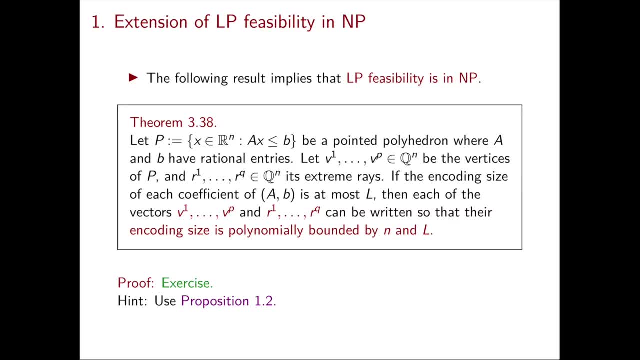 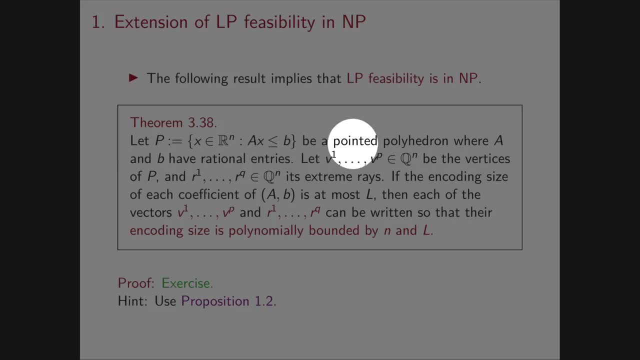 So let's read through this theorem. We have a polyhedron here, so there's no integrality at all in this theorem. We have a polyhedron, ax less than or equal to b, pointed Everything is rational. Let's denote the vertices of P by v1 until vp and by r1 until rq- the extreme rays. 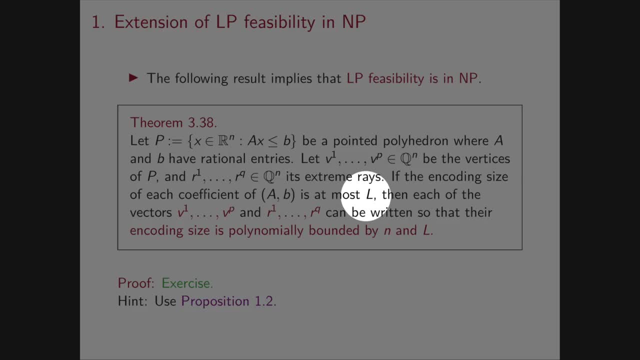 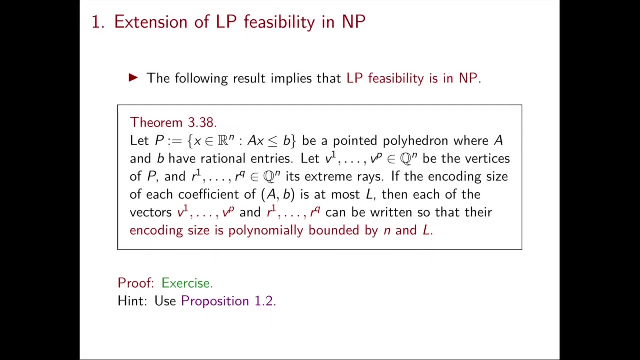 Then if we use again a-prime capital L to denote the encoding size of every coefficient of a and b, then every vector v and every vector r can be written with encoding size polynomially bounded by n and l. So once again, if we only think about the v's and forget about these r's, 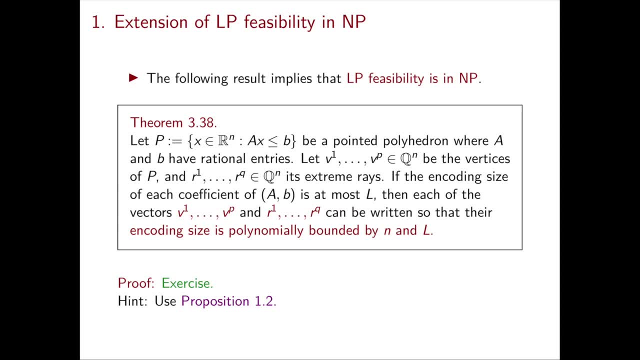 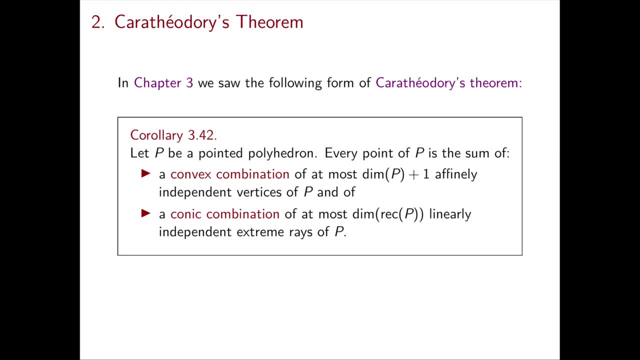 this is exactly what we saw to show that linear programming is in NP. So here it's a little bit more than that Good. So then the next result that we want to use is Carathéodory's theorem. Here I just copy-paste the result we've seen back in chapter 3,. 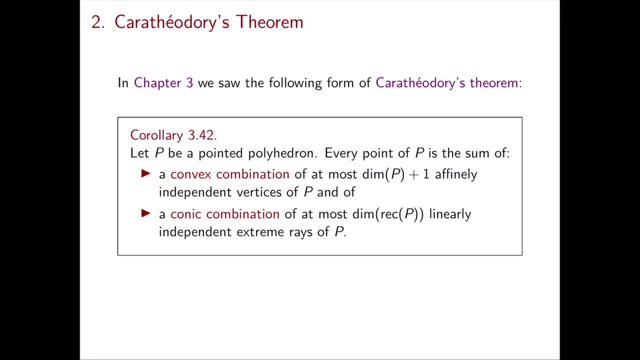 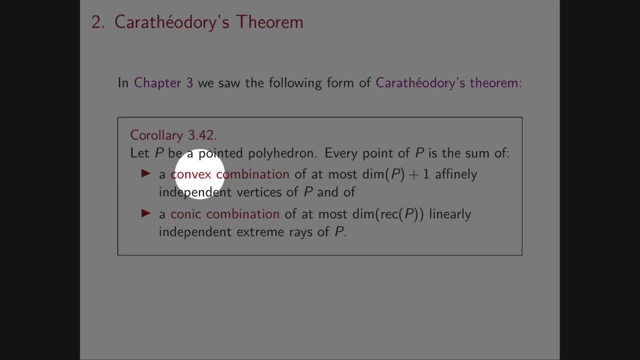 which is the most general form of Carathéodory's theorem. If we have a pointed polyhedron P, then every point in P can be written as the sum of a convex combination of at most dp plus 1 affine independent vertices of P. 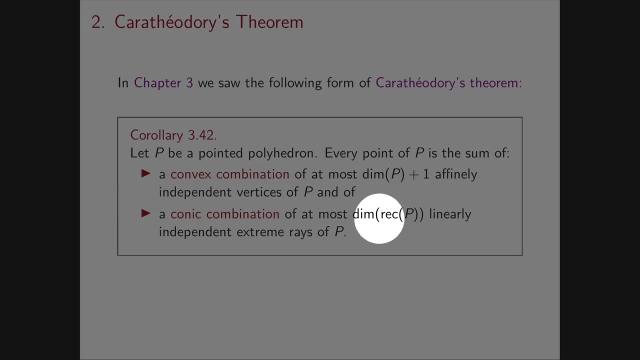 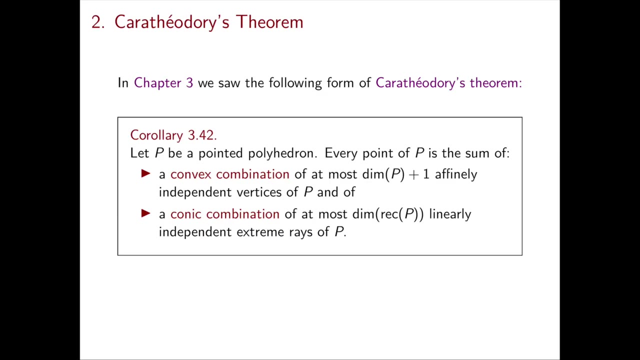 and a conic combination of, at most dimension of recession: cone of P, linearly independent extreme rays of P. Just a reminder so that, because we're going to use it very soon, Great, At this point we're ready to prove lemma 4.35.. 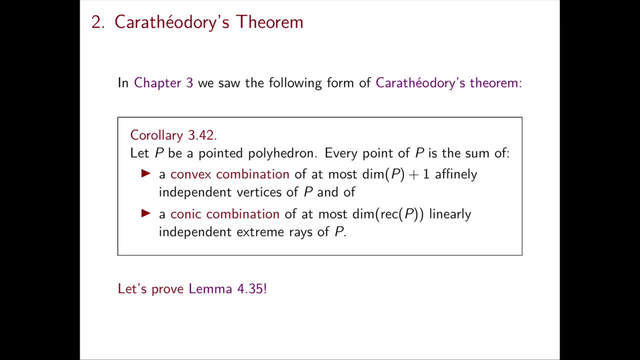 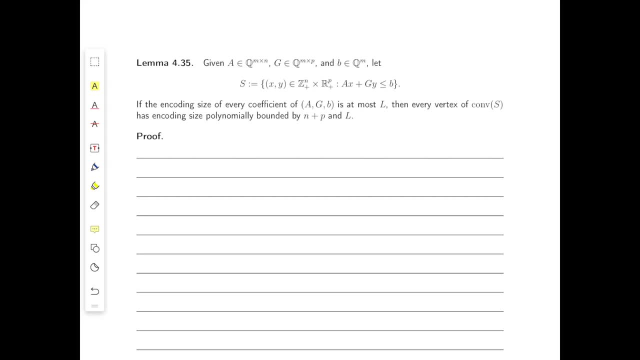 So let's switch to the notes. So here is the statement, And so what's the idea? We want to look at our polyhedron P, defined, as always, as a set of points satisfying Ax plus Gy, less than or equal to P and no negativity. 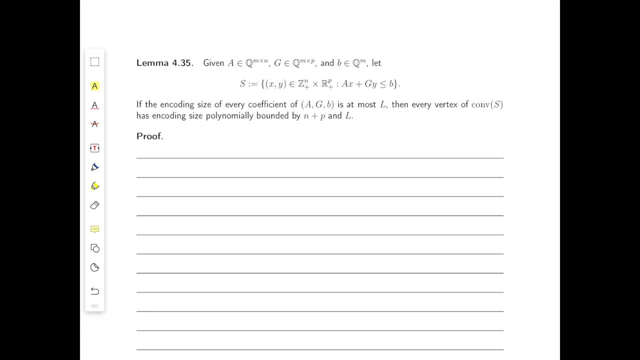 So just a linear relaxation of S, And the first thing we want to do is apply our extension of linear programming feasibility to this polyhedron so that we can obtain that all the vertices and all the rays are F-polyhedron. So this is just a set up, essentially. 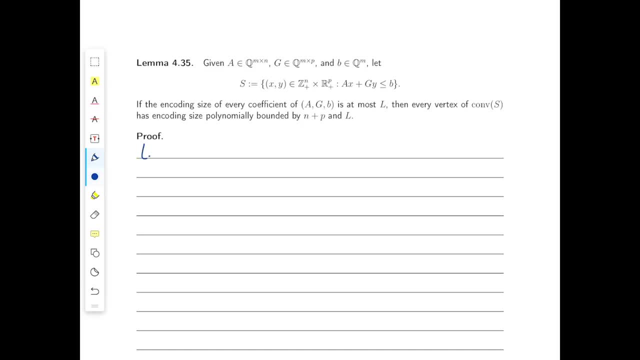 Let's write it down. Let P be the set of points in Rn plus times Rp plus, such that Ax plus Gy less than or equal to P. Then let V1 until Vt be the vertices of P And R1 until Rq be its extreme rays. 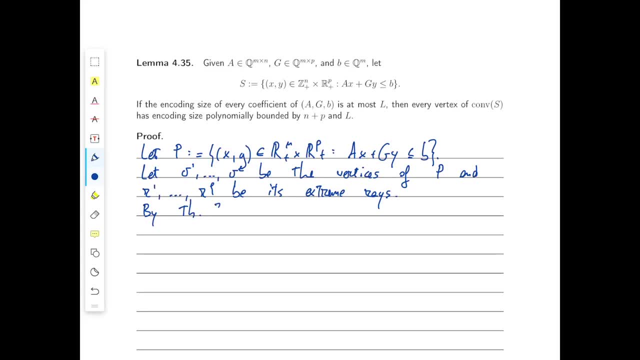 So by theorem 3.38.. All the Vi and the Rj can be written so that their encoding size is polynomially bounded. So we can write this integral by N plus P and capital L Also. on top of that we can always rescale our rays. 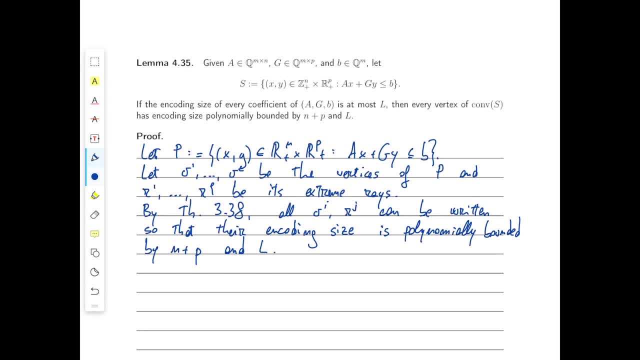 so that they're integral. And again we have seen back in chapter one that the size remains polynomial in N plus P and L. So bye, remark 1.1,. we may assume All are J. Okay, so our next task is to simply use Carathéodory's theorem. We pick a vertex of converse which 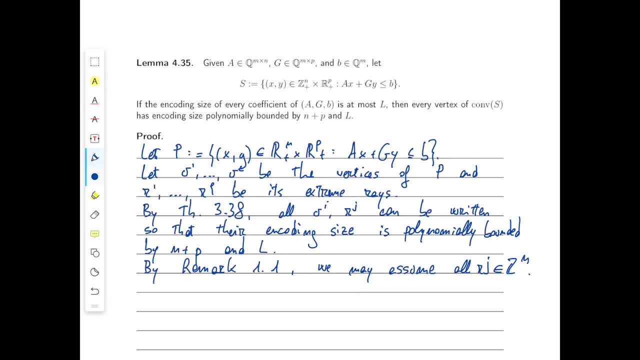 remember is: what we want to show is our certificate, what we want to show that has small size, and we use Carathéodory's theorem to write it as a convex combination plus a conic combination of few of the vi's and few of the rj's. So let's do that. 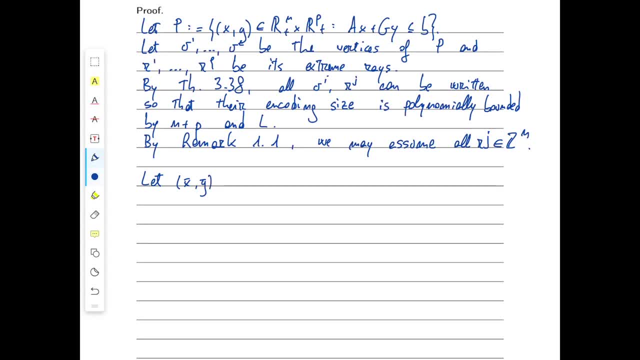 x bar y bar be a vertex of converse. Since x bar y bar is in P, by Carathéodory's theorem, x bar y bar is in the convex hull of only n plus P plus 1 vi's, without loss of generality. 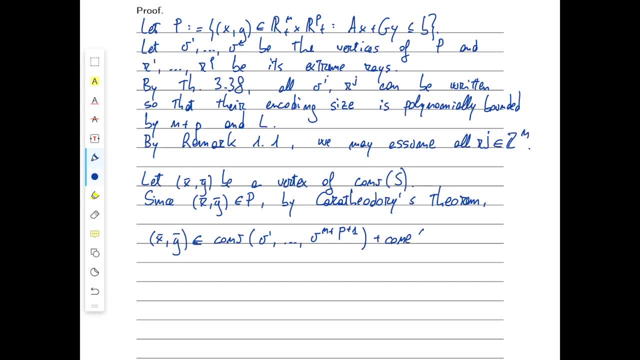 the first ones, plus the con of only x, bar y, bar n plus P of the ri's or rj's, And, again, without loss of generality, just the first n plus P, And so let's call this new set Q, which of course is a subset of P, And let 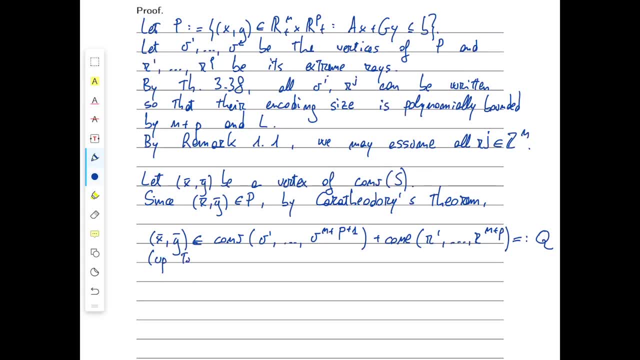 me just note here up to reordering the vi and the rj's. Okay, so I just mentioned that Q is a subset of P. So since x bar, y bar was a vertex of the feasible points in P, it will also be a vertex of the convex hull of the feasible. 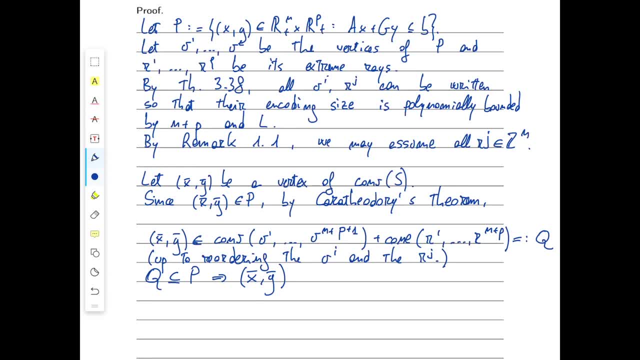 points in Q, since that's just a subset and this point is still there. Thank you, So is a vertex of converse: Q intersected z n times r, P. Okay, so good, Now we have somewhat set up what we needed in order to now use the proof. 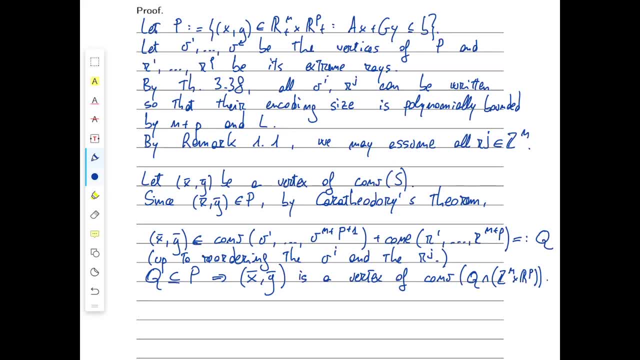 of Mayer's theorem. Remember I told you that this proof is a set of P. This is essentially a modification of Mayer's theorem, of the proof of Mayer's theorem. We just need to use two ingredients on top of that pretty much, and we just use both. 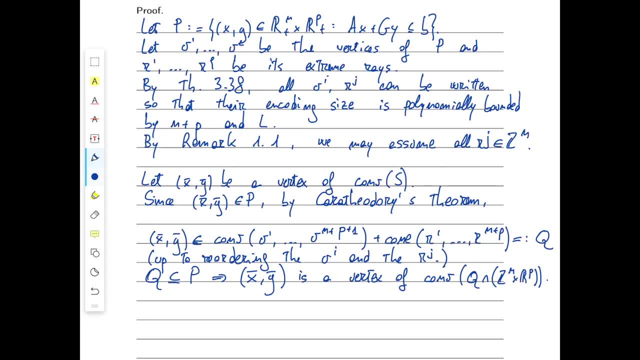 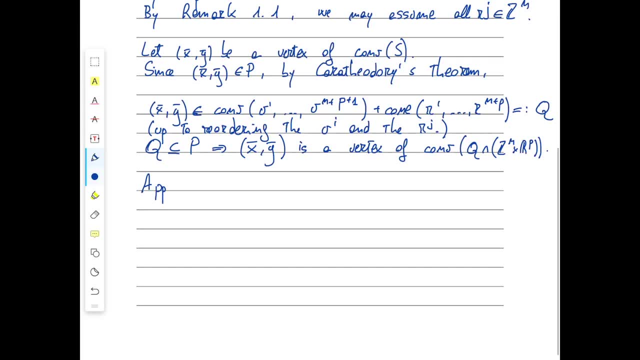 of them. First we use this extension of LP is in MP, and then we use Carathiodorus' theorem. So what we want to do now- let me write it- is applying the proof of Mayer's theorem to Q. So what do we obtain? 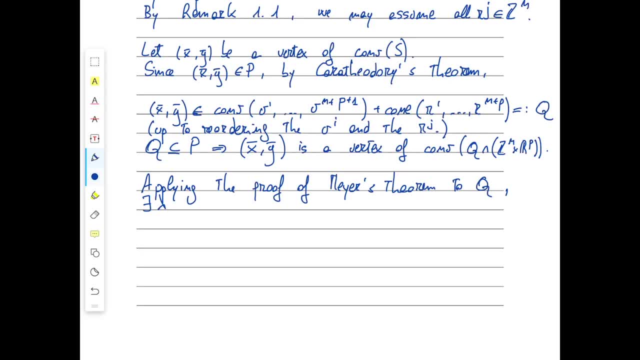 That there exists, so we're looking at the truncation of Q, So let's write it. There exists lambda greater than or equal to zero sum for i equal one until n plus p plus one of lambda, i equal to one and zero. 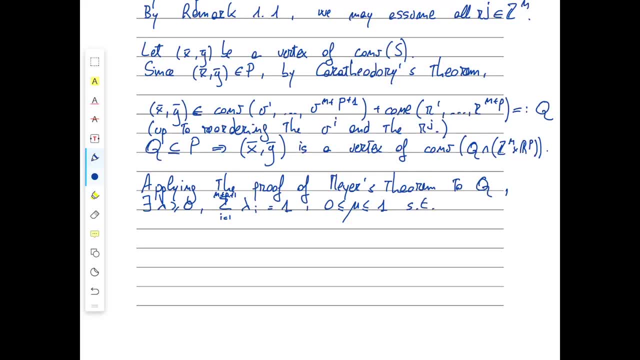 new one such that the vector x bar, y bar is in this truncation. This is exactly what we did in the proof-of-Meyer theorem. remember this holds because this point is a vertex of the convex hull of the points that are feasible. and in Q 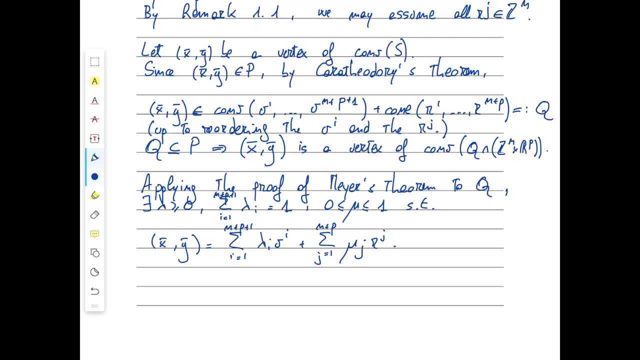 Good. So now, essentially, this equality already allows us to show that the vector x bar has polynomial size y. so if we denote by theta the largest absolute value of an entry In the vectors vi and rj, it follows that the absolute value of x bar i is upper bounded. 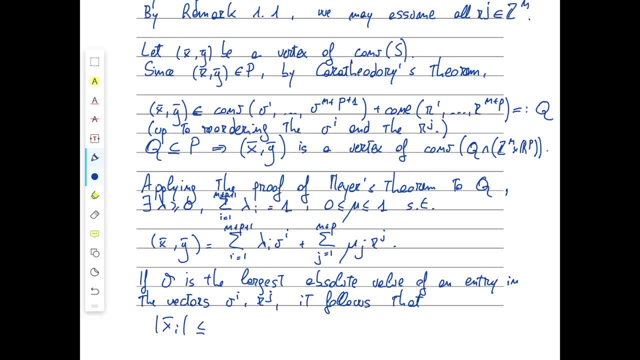 by what? So every entry? so let's look at the above inequality. Every entry of vi is upper bounded by what? So every entry of vi and rj is at most theta. so what happens with the multipliers? Well, every mu j is at most 1, and the sum of all the lambda i's is at most well it's. 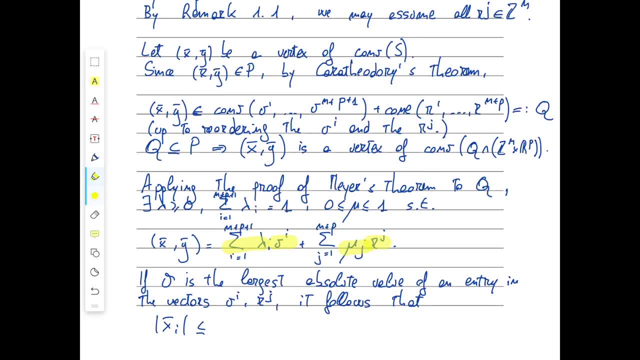 exactly 1.. Therefore, we obtain that this absolute value is upper bounded by theta, oh sorry, by theta, which multiplies 1 from the lambda i's, And this happens for every i equal 1 until n. Perfect. So we know at this point that x bar is an integral vector and its absolute value is: 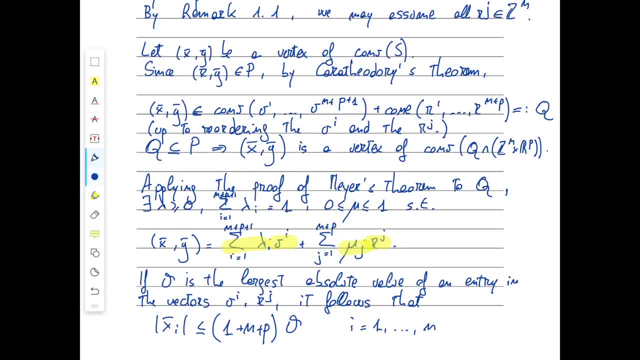 bounded by this number, which is a polynomial in n plus p and theta. so we're done, Let's write: So we're done with x bar. Since we're done with x bar, since we've broken the integral value, we're going to take the. 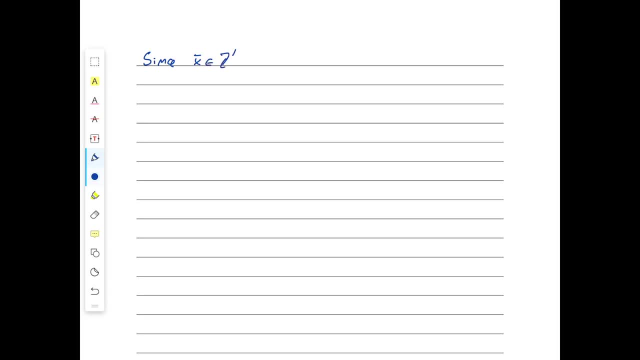 absolute value of x bar. x-bar is integral. its encoding size is polynomially bounded by n plus p and L, which is what we wanted. Good, so at this point we're done with x-bar. why are we not done with the y-bar? The same argument, in fact, applies. 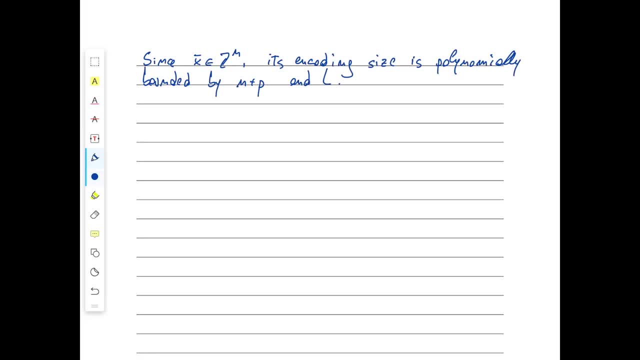 the only difference is that y-bar might be not integral, so therefore y-bar still can be upper bounded in the same way, but it can be- I don't know one, you know- like a very small number, one over a number that is non-polynomial in n plus p and L. 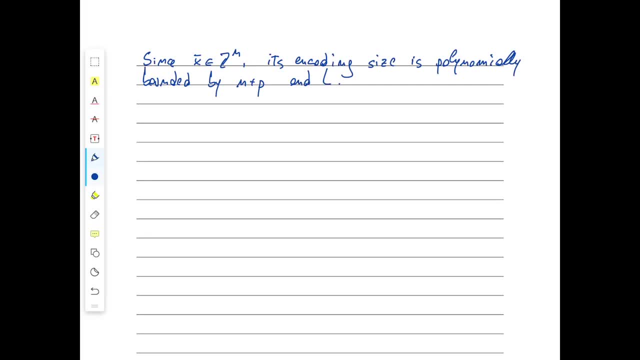 therefore, we cannot argue that the same thing for y-bar that easily. we need a little bit of a better argument. So, and what we're going to use is the following: the idea is the following: that pick your x-bar, y-bar, and now look at the polyhedron obtained from p by setting x. 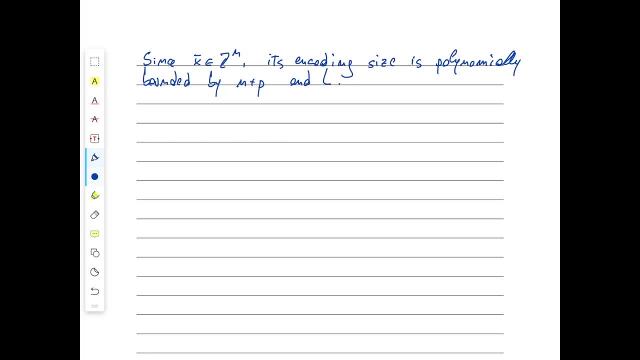 equal to x-bar. so essentially you take a slice of this polyhedron only in the y space, so you obtain just a polyhedron in the y space. Now the point y-bar will be a vertex of this new polyhedron and therefore 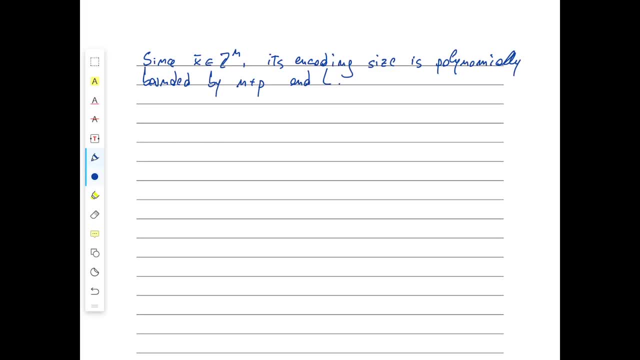 we can use again essentially the result that every vertex is of polynomial size in a polyhedron and conclude our argument. So let's write step by step what we have to do. So first, x-bar, y-bar is a vertex of converse, which implies: 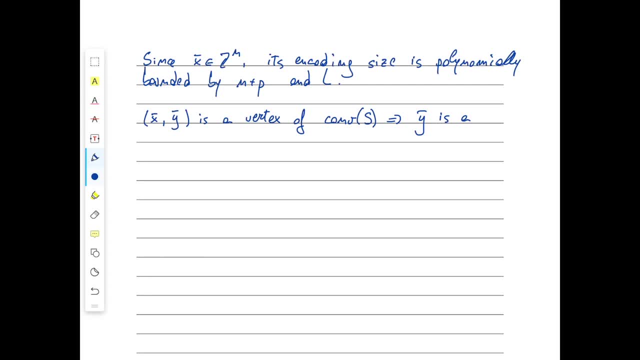 that y-bar is a vertex of converse. So let's take one vertex of the polyhedron y in r plus p, such that gy less than or equal to b minus ax-bar. so we are fixing x-bar. Now what is the data in this polyhedron?